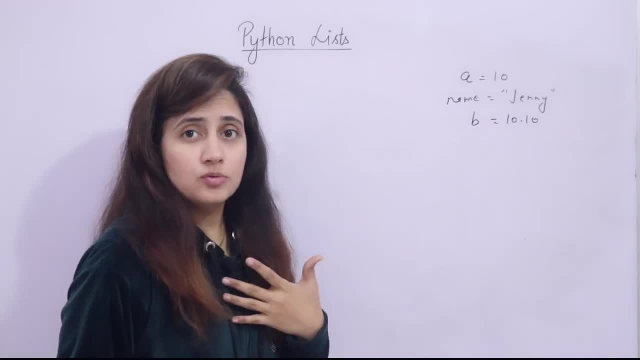 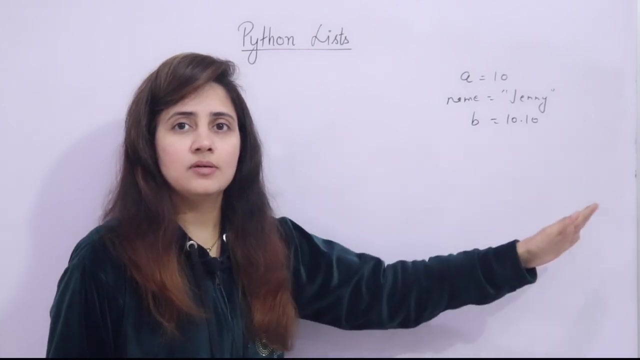 But the problem is, if I want to store, suppose in my class I have 15 students, So I want to store row number of 15 students. So one method is what The method is still now we have discussed is what We can create: 10 variables: a, b, c, d and in individual. 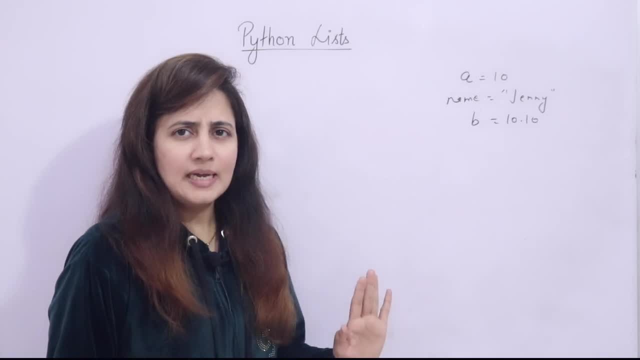 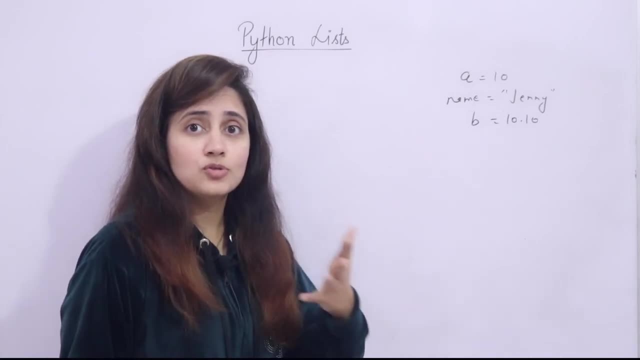 we can store 1, 1, 1 row number, right? But that is, I guess, not a good idea, right? If suppose I want to store. in my class I have 60 students, So I want to store row numbers of 60 students and names. 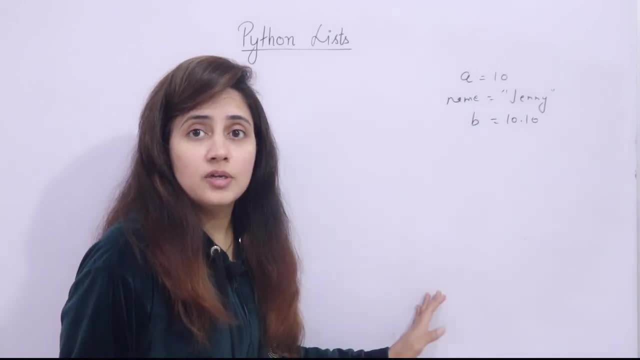 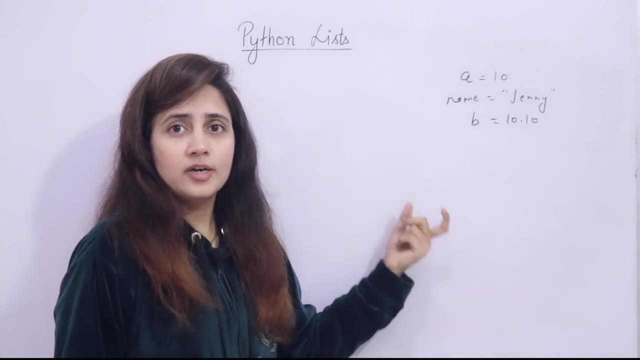 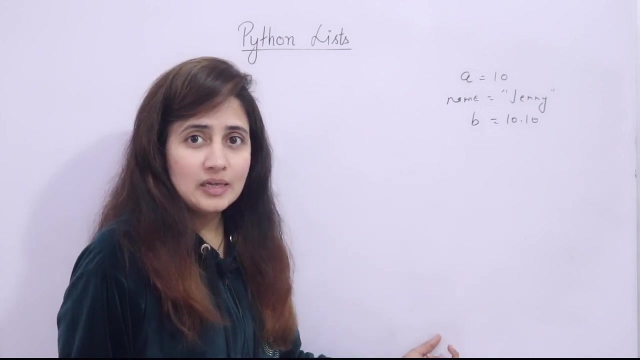 of 60 students, Then you have to create 60 variables, right? Because in one variable we can store only one value, right? But I guess that is not a good idea to create 60 variables to store 60 row number of 60 students. That would be very time consuming, length you know code would be very. 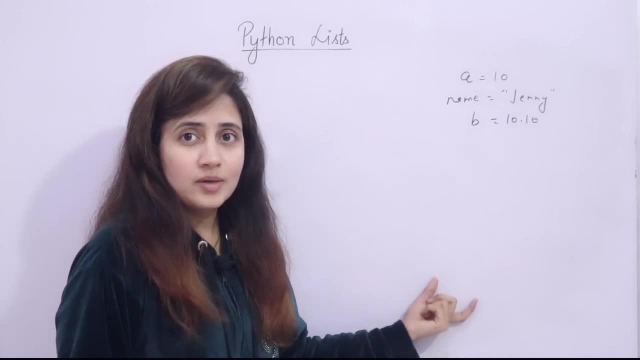 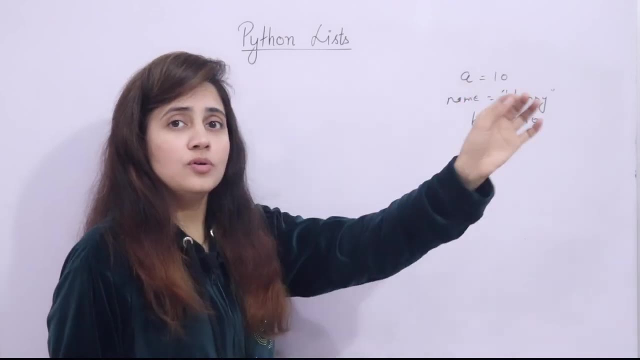 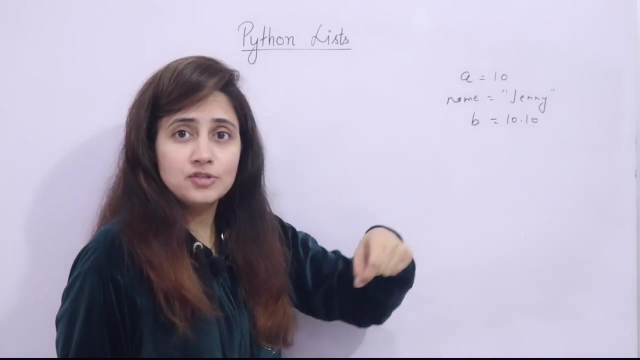 lengthy and error prone code would be there that was not readable. many problems would be there. So is there any way under a single variable name we can store row number of 60 students, Row number of 10 student or 60 students or 100 students under a single variable name? Yes, we can. 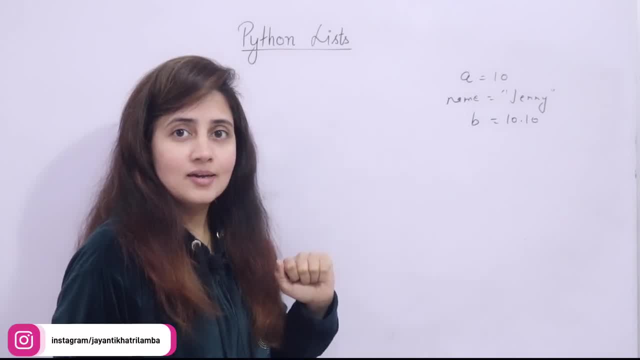 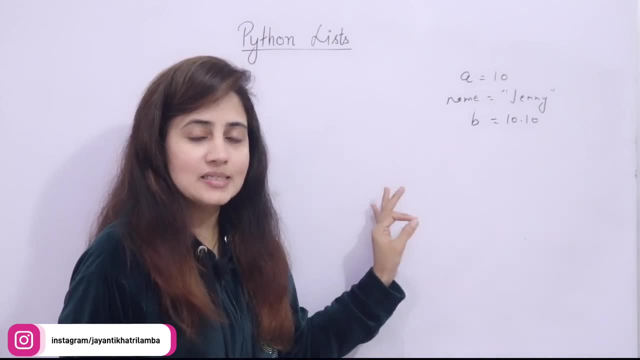 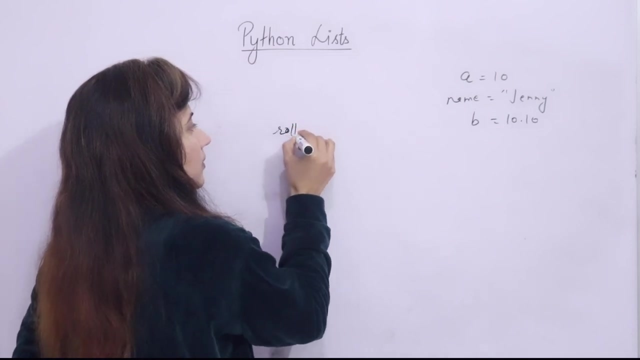 do with the help of list right. There are other ways, also in python, tuple set dictionary. those also will be discussing one by one in later video. but here we will be discussing list right. So what we can do, I can create some simpler variable. suppose I am taking row number right And there I 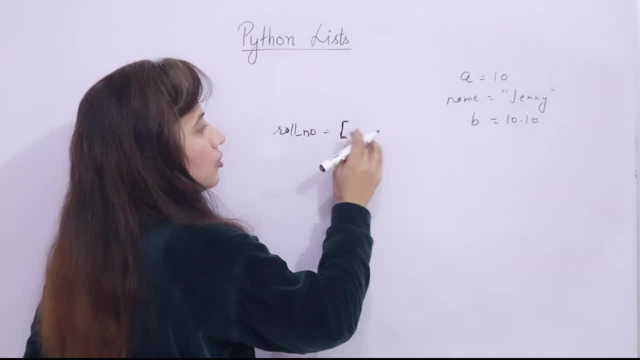 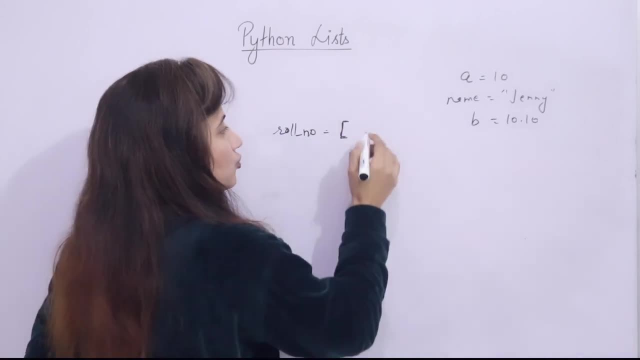 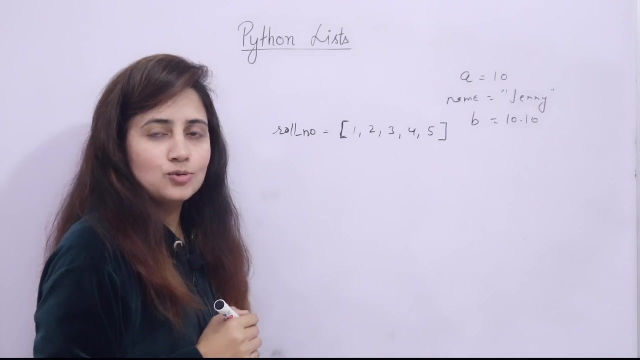 can store these square brackets. opening brackets, row numbers of 5, 10 or 50 or 60 students- as many students as you want. like I am taking only five students: 1, 2,, 3, 4, 5- and closing square bracket. that is it. So this is what a list right Under a single. 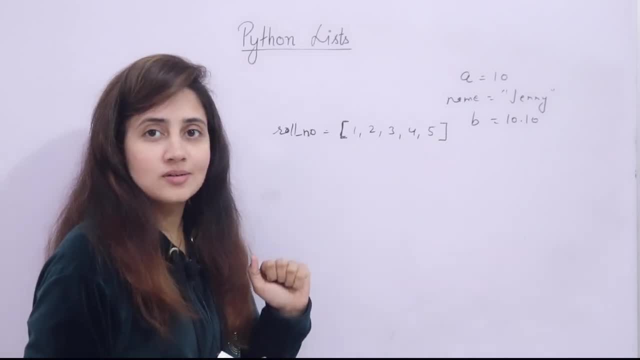 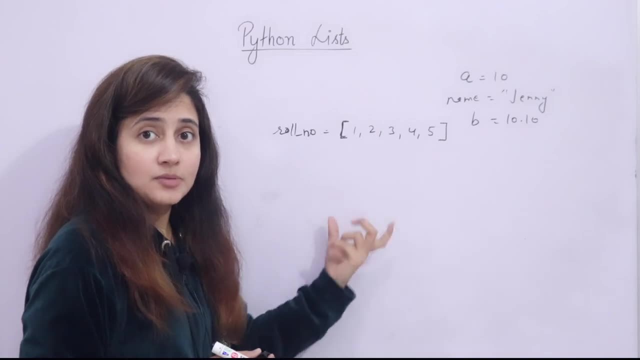 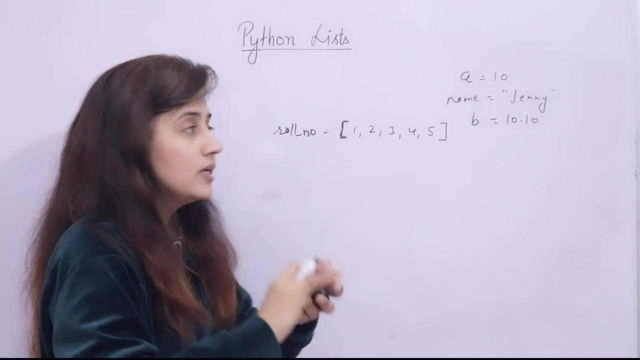 variable name. we have stored these row number of five students. So basically, this list is what It is: a data structure. It is just a way of storing and organizing the data. It comes under sequence data type Because contains sequence of you know types of data. and see if once list I am creating. 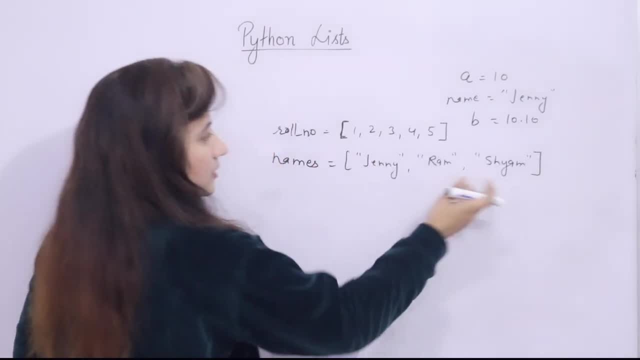 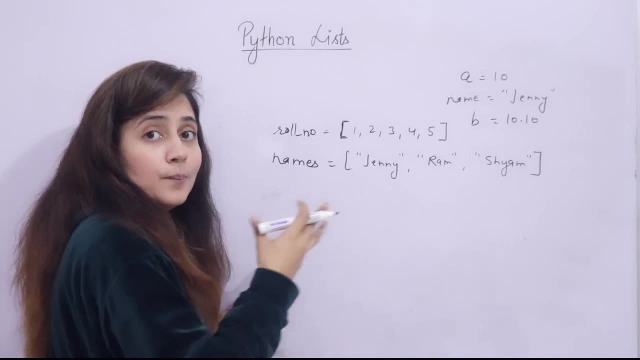 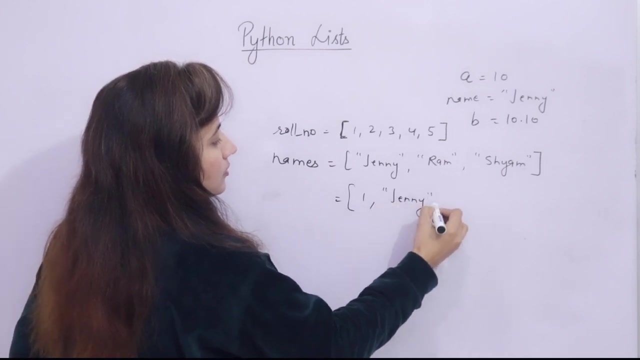 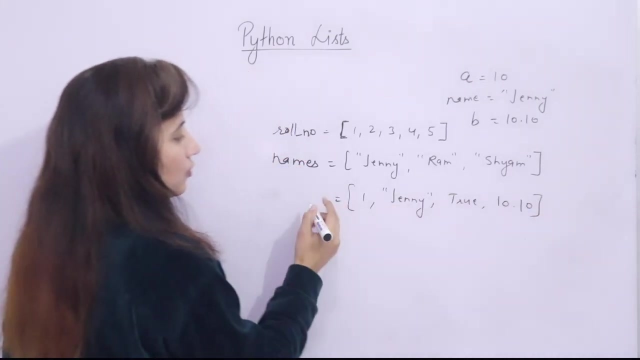 for names. names is equal to like this. so this is, these are strings, these are integers. right, but we can have mixed type of list. suppose in one list I am taking one integer and one is string, one is true force. these are Boolean data type, ten point one, zero. this is float. so suppose this: I am taking mix, underscore. 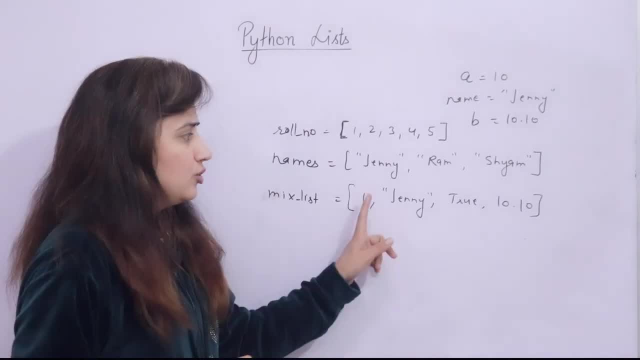 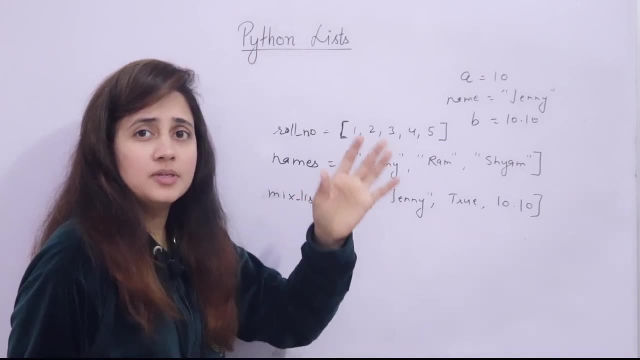 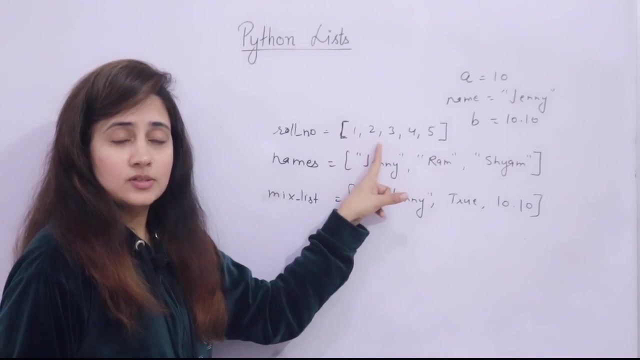 list. so this is also allowed. collection of different, different data types also allowed. same data type also allowed. like if you have at the array concept in C, then array is what? collection of similar data type, homogeneous, right. so if this integer, integer data you want to store, then one array you can store only. 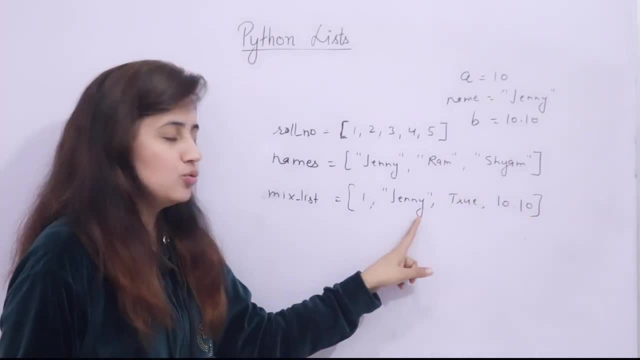 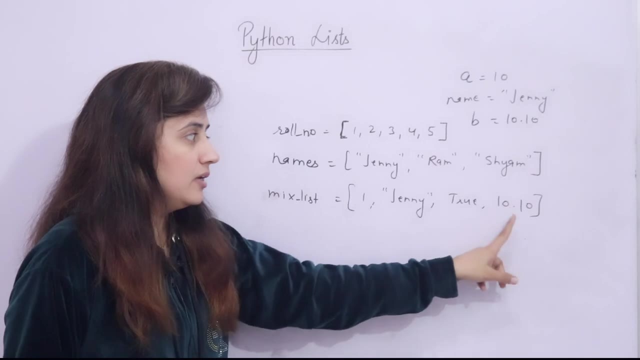 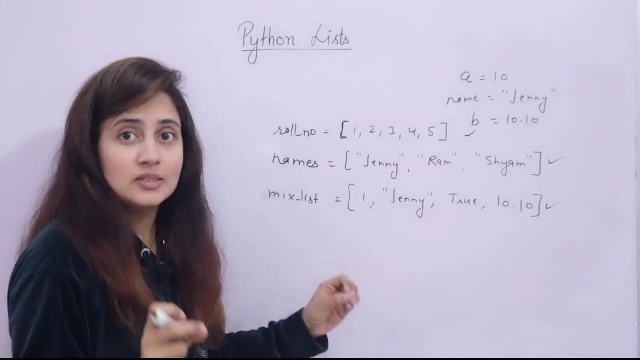 integer types of data only. it's not like that. this you- this is allowed. no, but in list it is allowed. a mix list is also possible. integer string, Boolean float: this is valid. list- this is also valid. this is also well. so this is, I think, very powerful tool of Python language. the list, and still there are many. 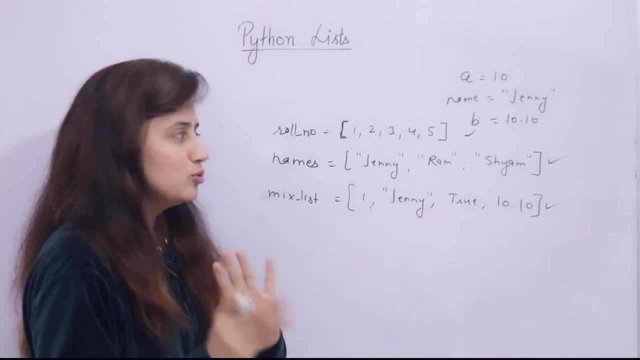 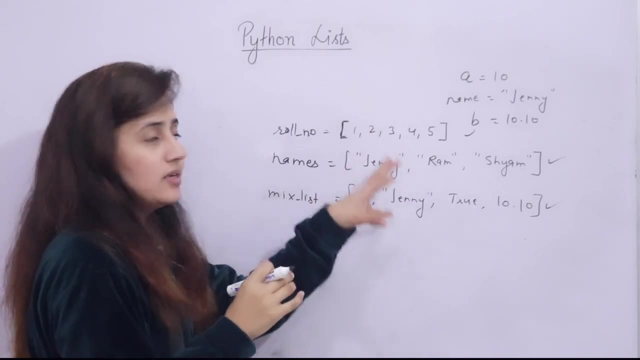 functions and many you know interesting things we can do with list. those also will be discussing. so basically, list was what. you can say it's a container or it's. you can take collection of things. you can say it's a container or it's. you can say collection of things. 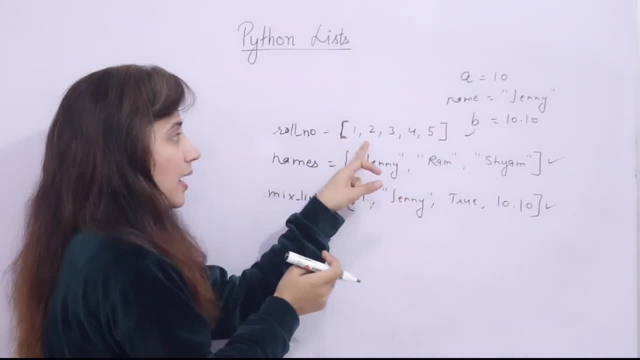 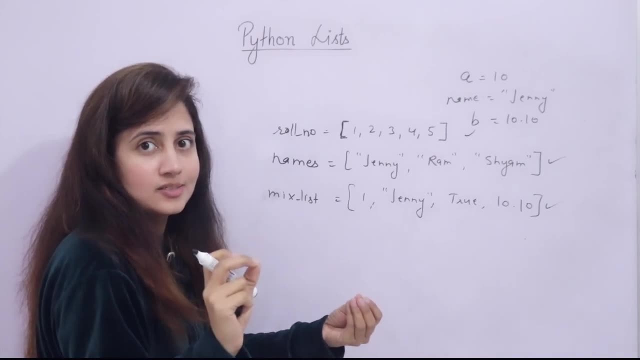 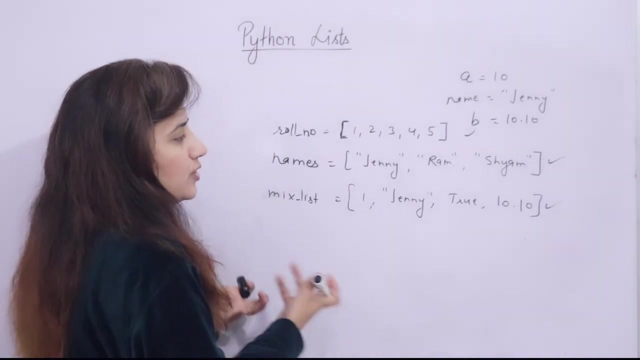 enclosed in square brackets and separated by comma. that is a list. It is. you can say it's a dynamically sized array, not fixed size array. dynamically sized array. we can say It's just a container, or you can say collection of things. and list is what? a sequence? data type, because 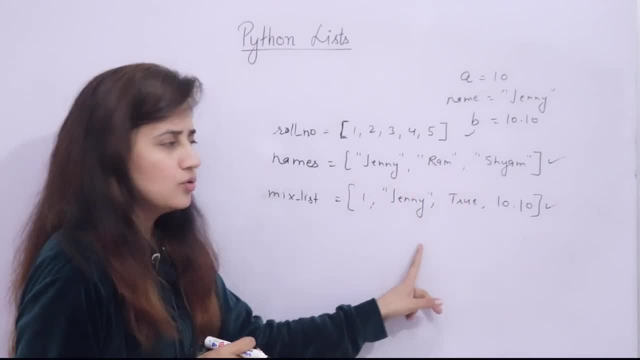 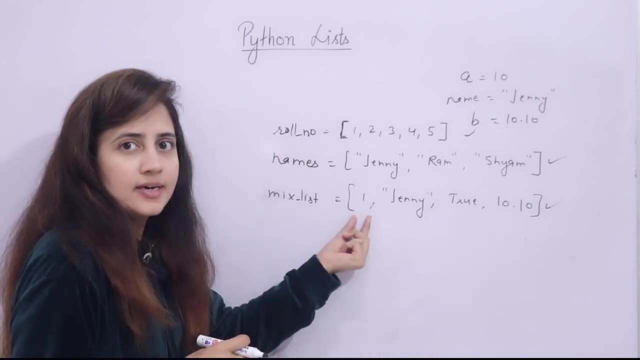 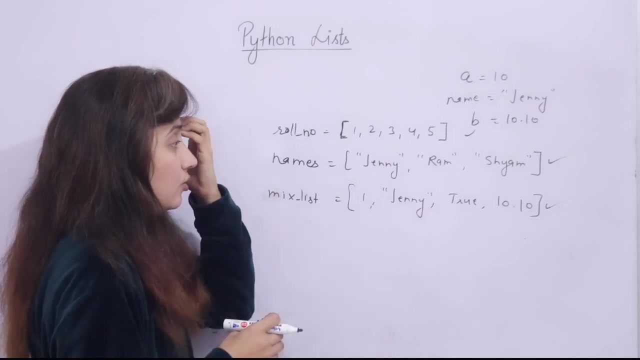 this is just a sequence of data. It is used to store sequence of various data types and it is not homogeneous. need not to be homogeneous, right? A single list can contain many data types, like integer, string, boolean, float and as well as objects. right Now some characteristics of list. 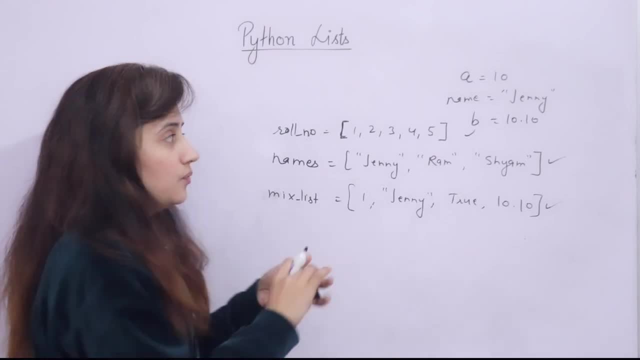 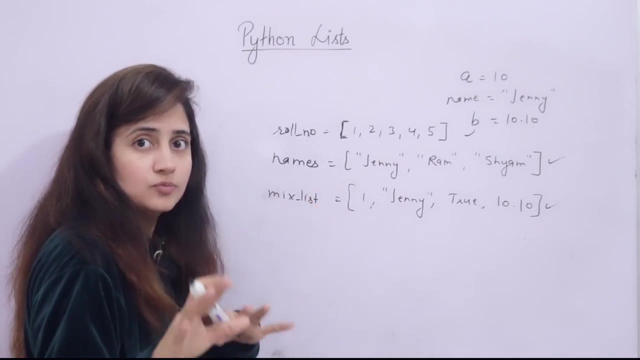 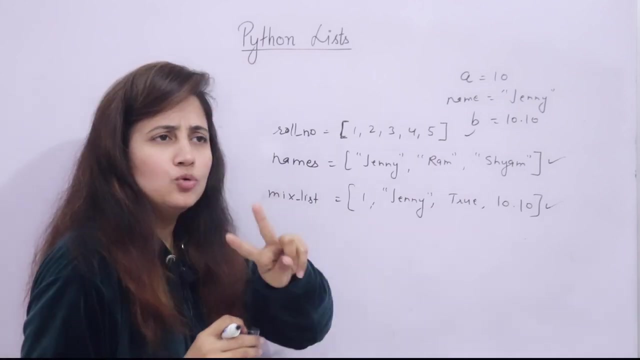 you can say like: but these are ordered, list are ordered. These items are having a defined order and these orders, this order of these items will not change right. One more characteristic is what these are: mutable. Two words are there: mutable, immutable. Simply mutable means, in simple words: 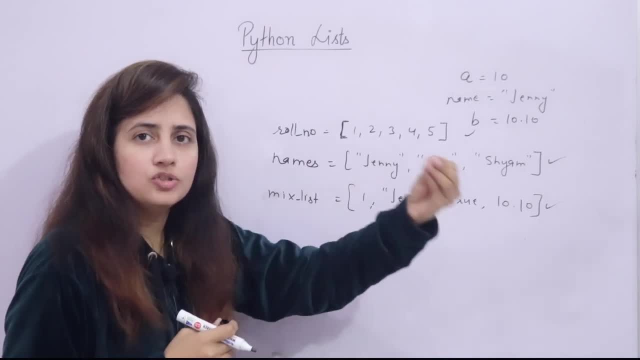 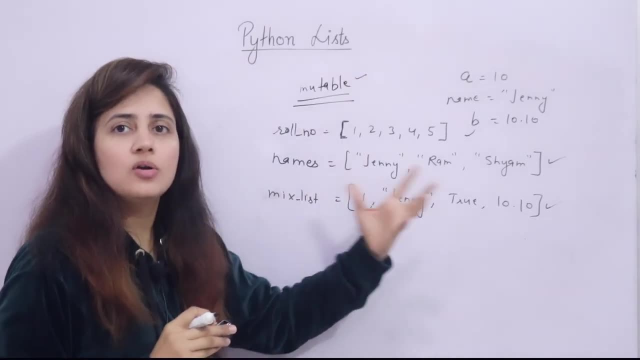 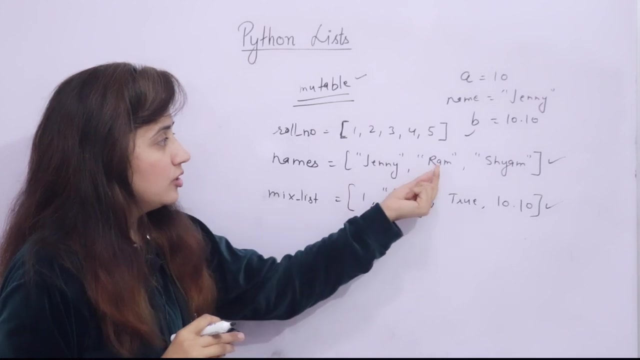 I am taking can change. Immutable means cannot change. Lists are mutable. Mutable means: after creating the list, we can alter the list, We can change the list. We can add some element, We can remove some element. We can, you know, change the here. suppose here I have Ram, We can change this name. I can do this Mohan, So this: 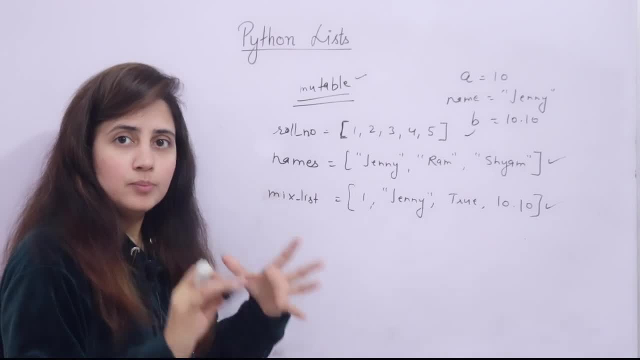 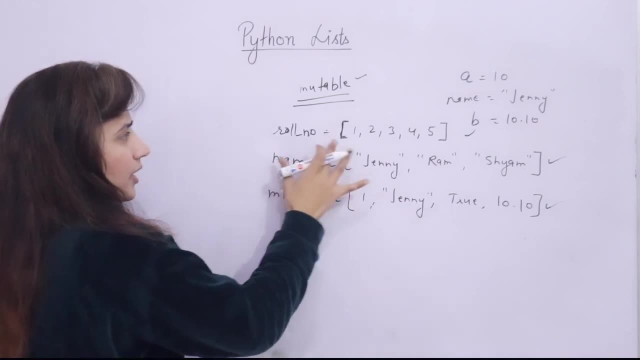 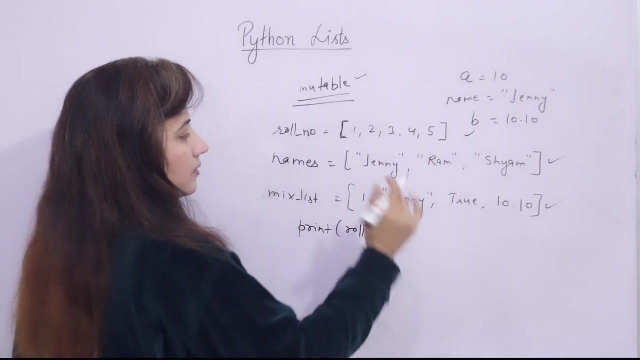 alteration is possible after creating the list. So lists are mutable, but lists are ordered. as well as how you can print the list now, If I want to print this row number, So simply print and name of the list, So it will print this thing. Output would be something like this: 1, 2, 3, 4, 5 in these square. 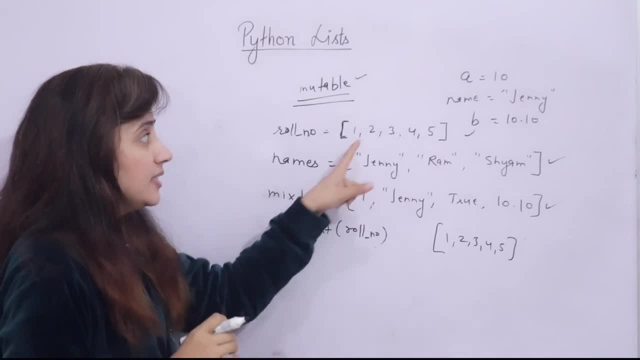 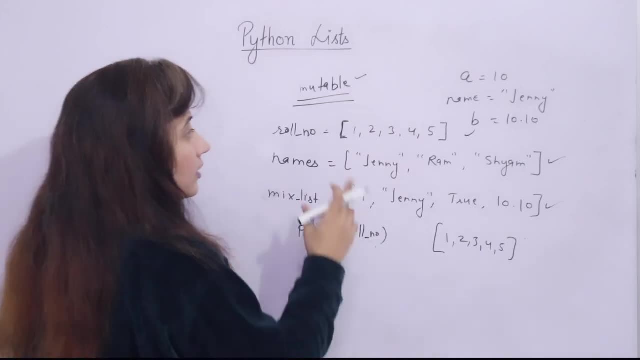 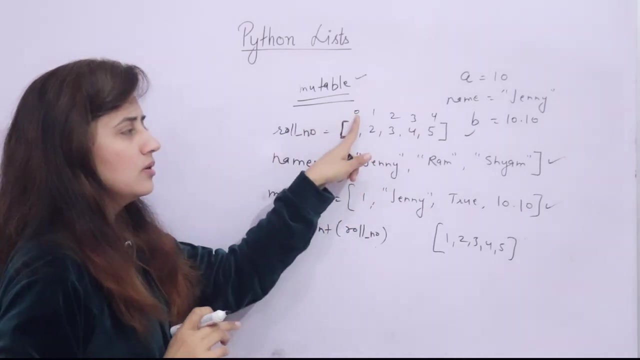 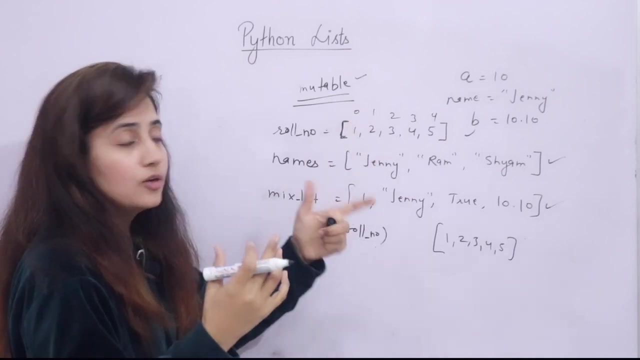 brackets, right, But if you want to access individual elements- suppose I want to access this 3- that is also possible using index. right Now, index is what Index of this is. index will be started from 0.. 3, 4.. Why this is from 0? It is not. you can say position, It is. you can say offset from the. 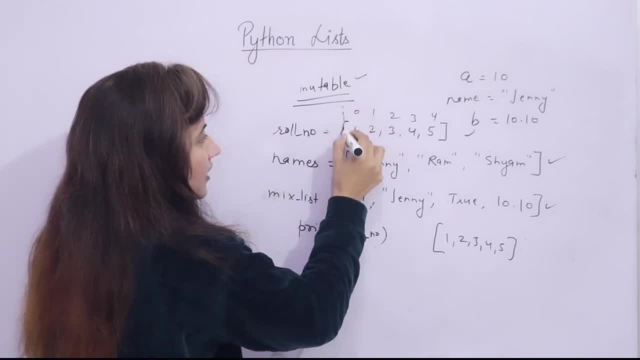 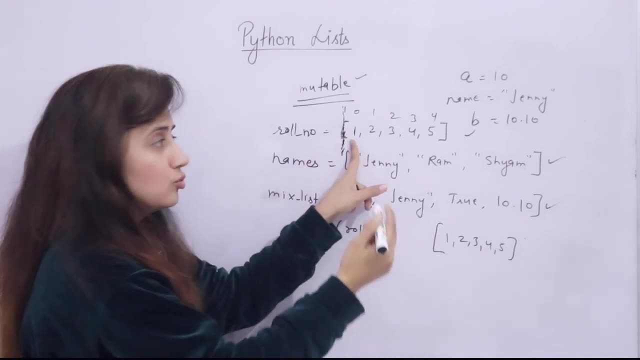 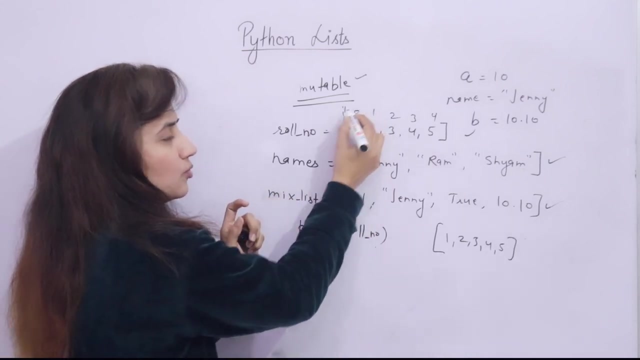 starting position. So from the starting position- this is starting position- you can say the shifting or offset of the variable. So offset of this variable from starting is what? Nothing, It is 0, or shifting is 0. So that is why index is 0.. 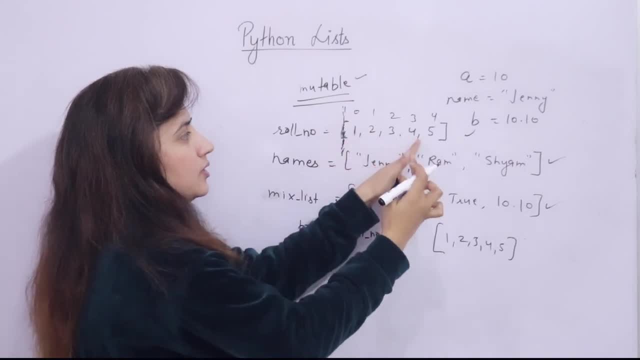 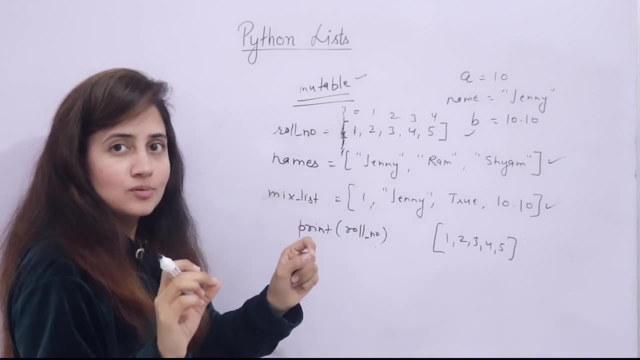 Shifting of this- This is from starting position- is 1, then 2, then 3, then 4.. That is why index generally starts in programming from 0. So for programmers, counting starts from 0, actually right. So using index we. 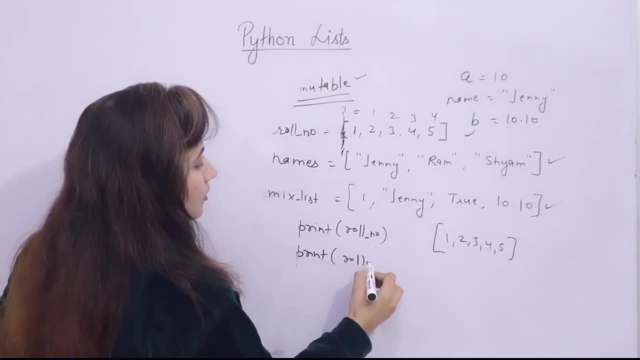 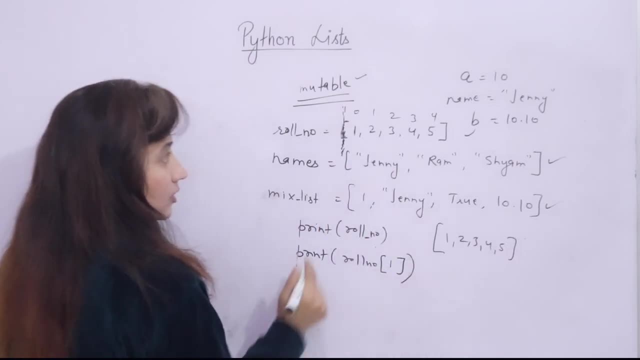 can access, like if I write print row number and in these brackets just put the index. Suppose I am putting 1.. So at 1 at this index, what is 2?? So it will print 2.. So it will print 2. So it will print. 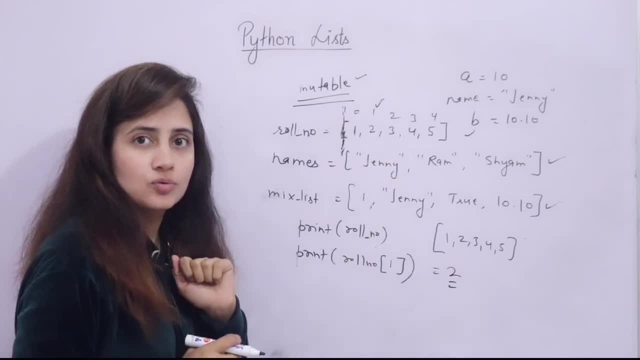 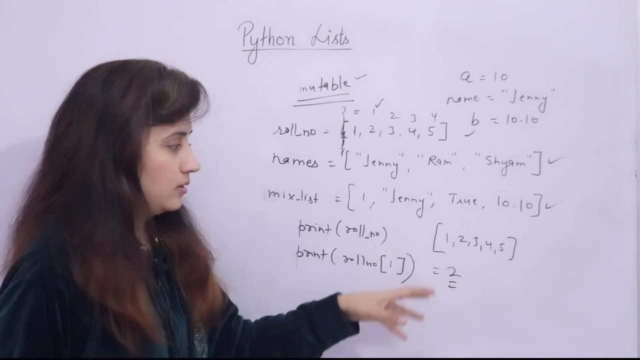 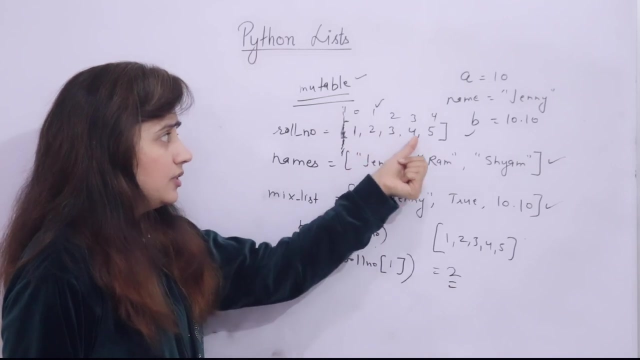 2. So you can access individual elements also. right, And many operation we can perform on list Like. we can sort the list, we can reverse the list, we can append more data, we can extend the list. right, We can count the occurrence of these items in the list. We can find out index of. 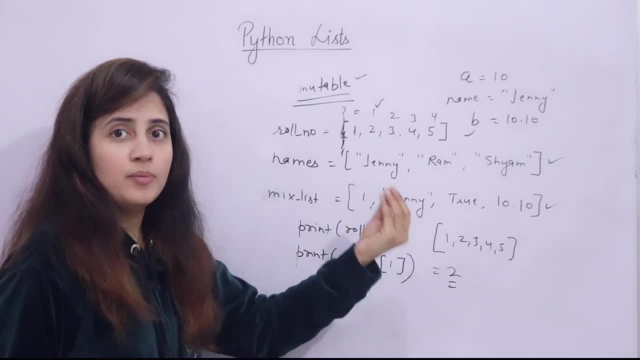 individual item in the list. You can find out length of the list, minimum or maximum from the list. Many methods are there, So those methods we will be discussing with the help of a program. I will see you in the next class. Bye. 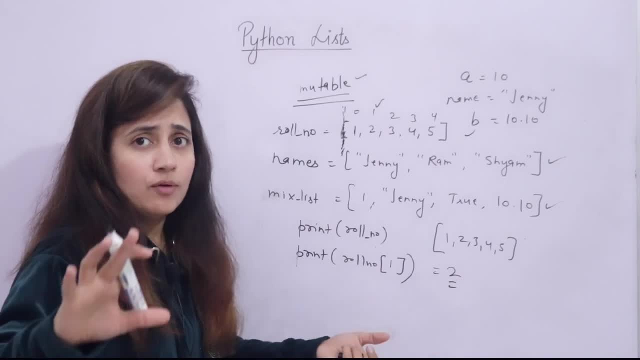 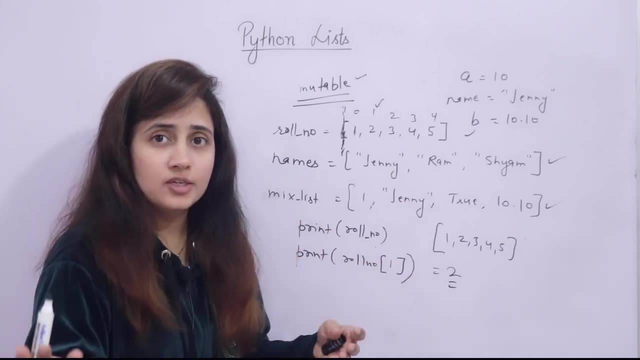 I will show you practically right, But you do not have to remember all the methods. Just take a look like everything is available on this documentation on the Google. when you see the Python documentation, Many methods are available, So you do not have to memorize all the methods. 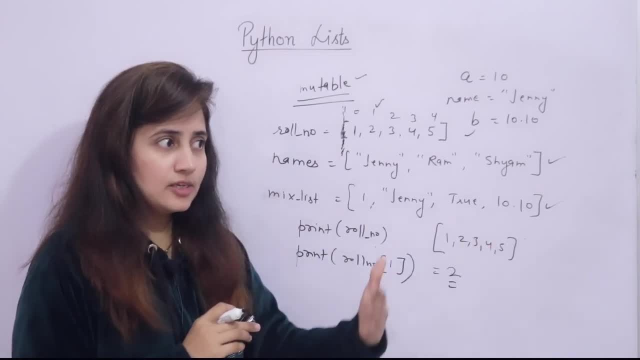 right, Just take a look how to. Yes, we can do this thing with list, we can do this thing with list. right, So that you have in your mind, yes, you can do, you can sort the list. There is a method. You do not have to write that thing, right, You just google. 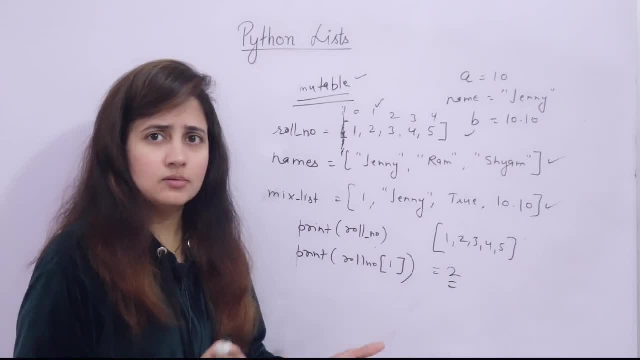 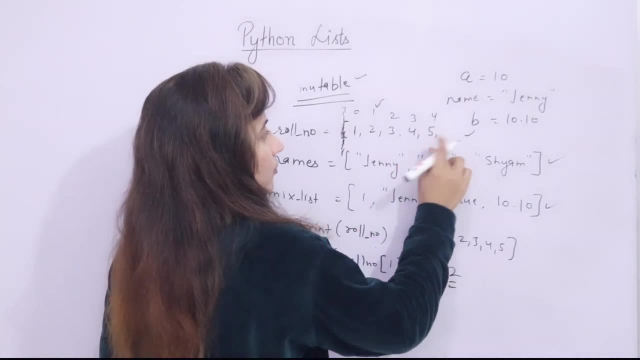 that method. how to you know? use that method. and that's it. and yes, one more thing in list. List can have duplicates value like five and comma more item. I want to add two comma one. These are duplicate, so this is a allowed in Set, actually, actually. 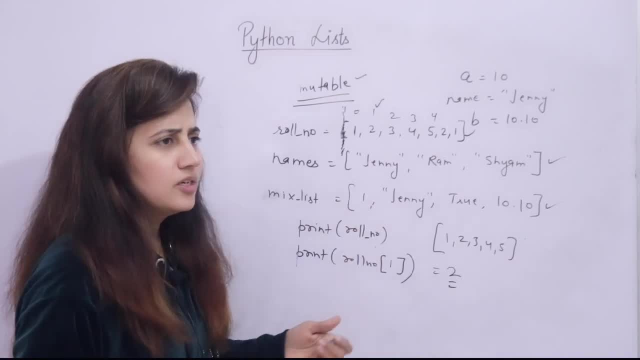 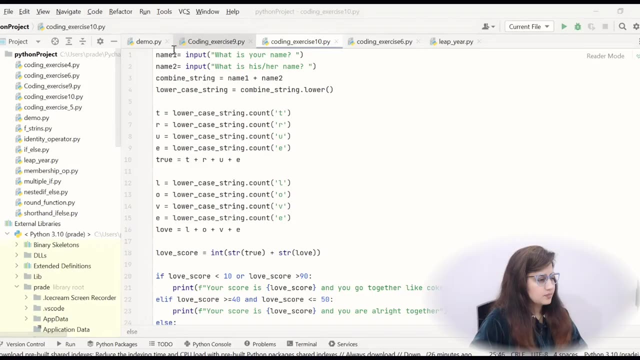 duplicates are not allowed right, But unless duplicates are allowed right. So these are some characteristics also of list. Let us see some functions of list. Let us create a new function. Let us call this as a switch. So let us create a new function on the list же. 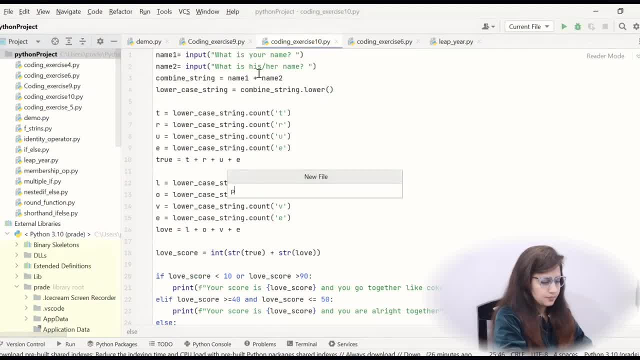 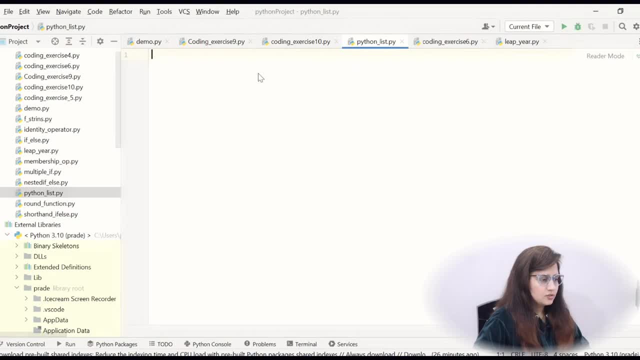 So let us create a new file, python list, dot py. right, and we will be taking first of all a list, suppose numbers. So suppose I have like only 4 elements: 10, 0, minus 1, 7, and if you want to print this, 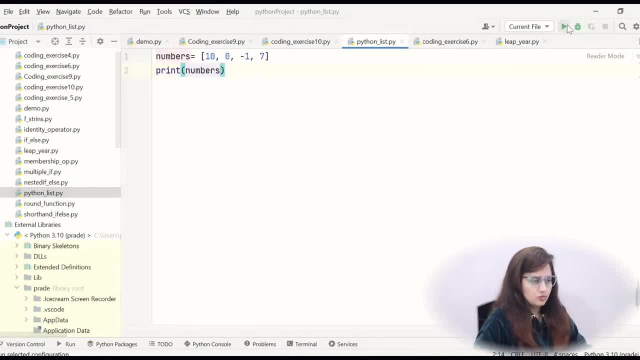 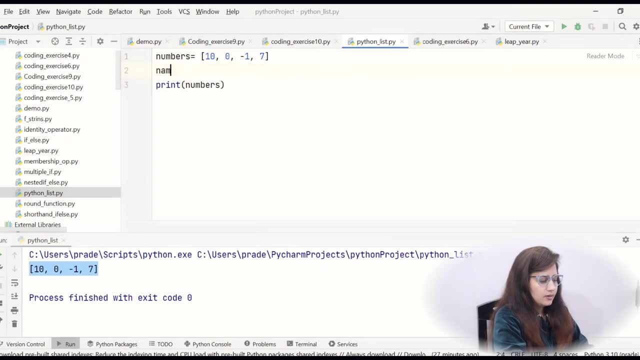 you can simply print, that is it? So let me just run this and it will print. see this thing with brackets, right, rather than this. if I want to store some names, that is also fine. you can store like this. if you want to store names, that is also fine. this is also fine. if you want to print, simply print. 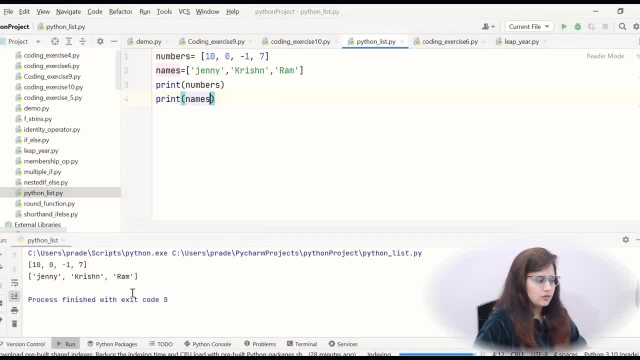 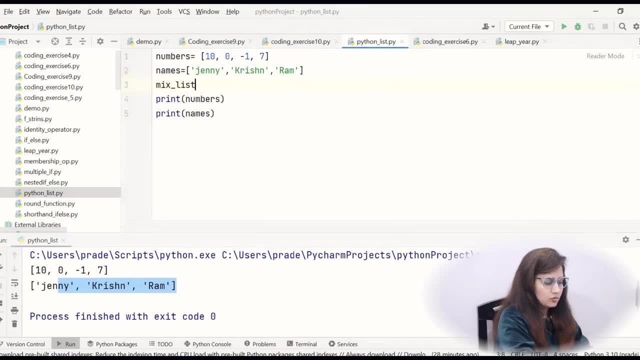 and names. So it will print this list also. right, as you can see, Mix list is also possible. like you know, If I take a mix, underscore list, a name and integer, then I am going to store like jenny, then I am going to store like true boolean data type and 10.10, something like this and 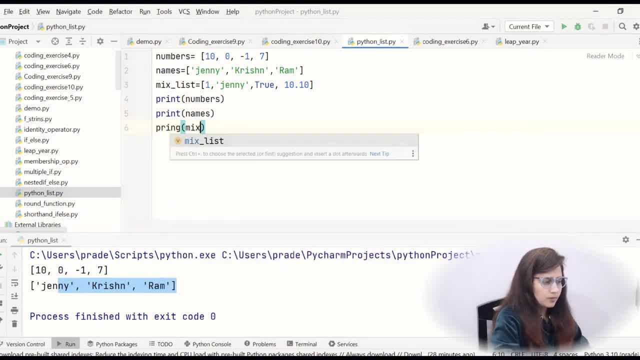 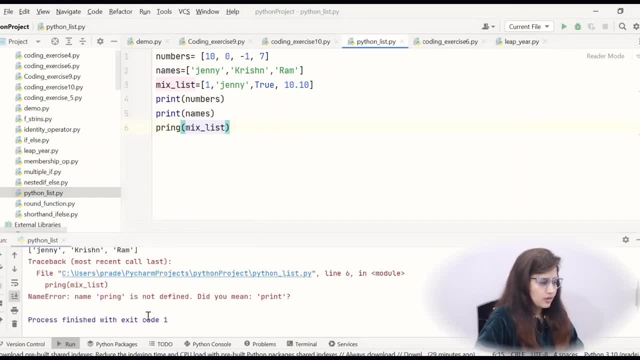 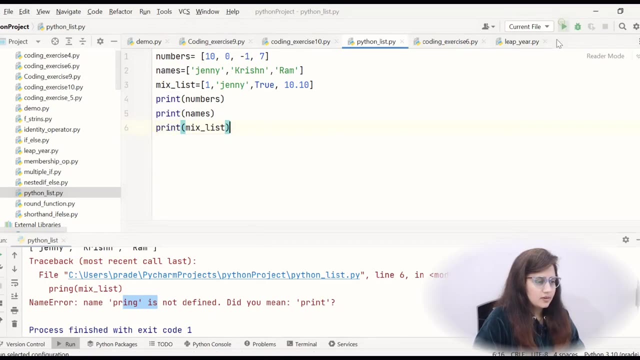 if I print this mix list, then it will print. ok, rather than this, we have an error like this: pring. It is print not p? r i n g, p r i n t right? let us run this So see it is printing this, so mix is also possible. but now let us come down to these. 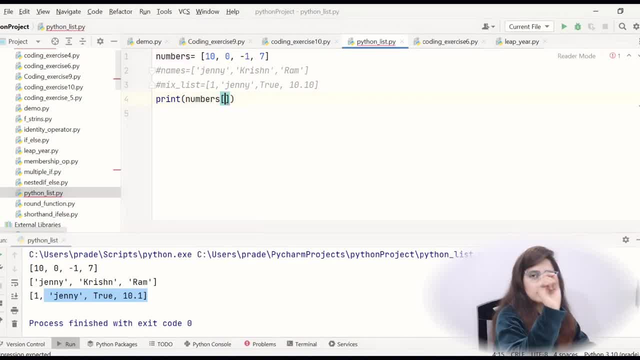 list and if you want to access individual using index individual- you know these items in the list- then you can access like number 1.. So now it will print what: 0, because at 1th index 0 is there rather than 1, if you will. 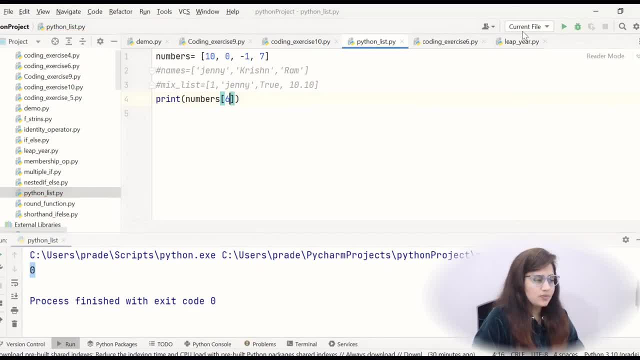 if you will write 6.. Ok, Obviously 6 is not in this list, the index 6, 6th right. So it will give error like list index out of range. So you can up to 0, 1, 2, 3, up to 3 index you can put. if you put 3 then it will print 7. 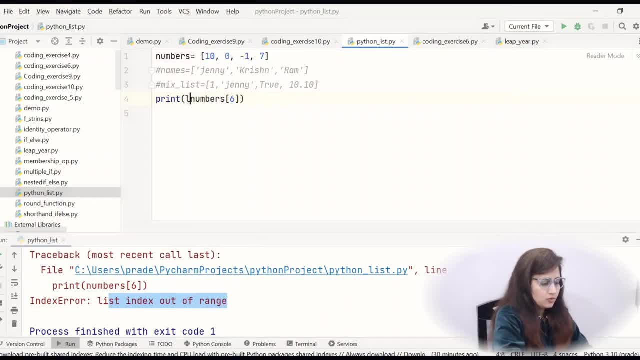 right. If you want to print number one function is like length. then you can simply use one function length and in bracket you can simply put the name of the list numbers. Ok, So see, length would be 4, 1, 2, 3, 4, right. 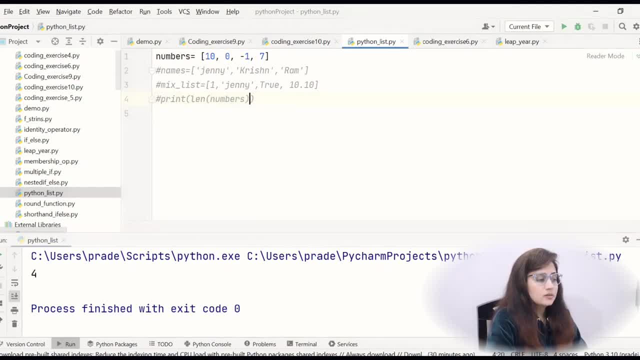 So this is what length. but if you want to access like, this is something called as slicing. but negative indexing is also possible. see, let me tell you print numbers. if I write minus 1, minus 1 negative index, start from backward. So minus 1 index is for this element 7.. 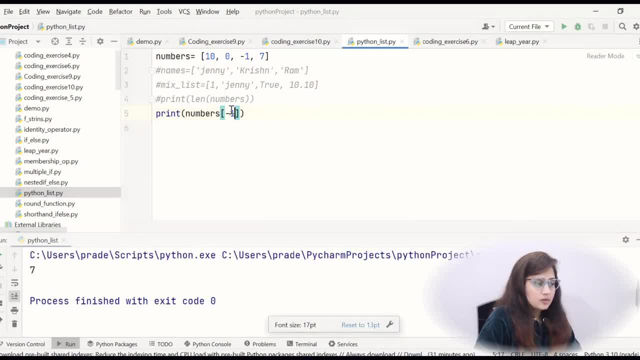 Ok, So it will print 7. see, if I write minus 2, then it will print minus 1.. So minus 1 minus 2, minus 3 minus 4, something like this. So backward negative indexing is also available in list. Now what is list slicing? see if I write something like this: starting index is 0 colon. what is? 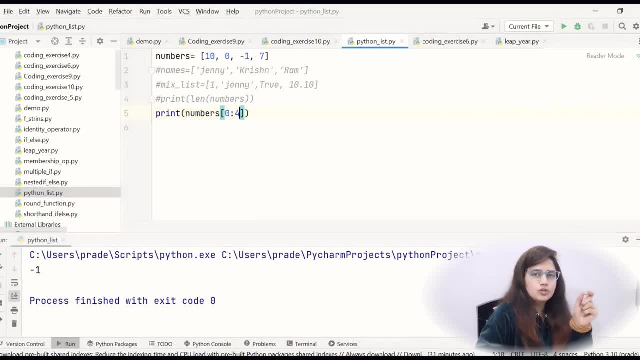 length of the list: 4.. So if I write 0 colon 4, it will print simple the complete list. Ok, If I do not write this, 4, just blank 0, nothing else. so by default it will take 4 here it will print the list. 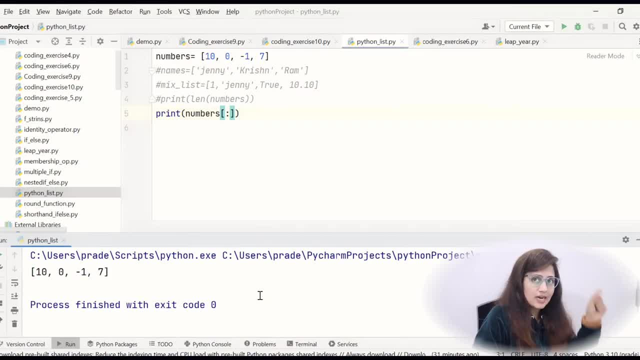 If I do not write 0, simply the colon. so by default starting is starting, point is starting index, ending point is length. by default these numbers are there, So still it will print the list. but if I do string slicing, if I write index, should be started from 1.. 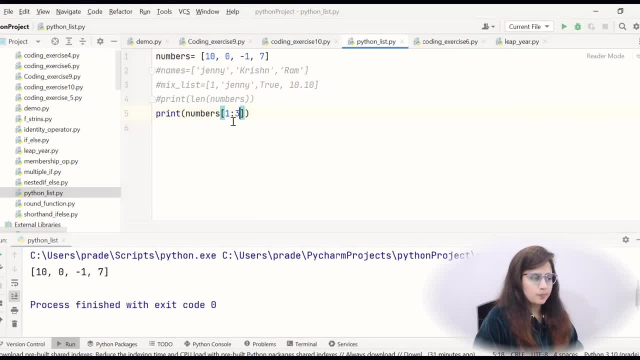 And 1, 2, suppose 3.. So 1 is the index, so 0 and 3 is what? till third length. So 1, 2, 3 mean till minus 1, so it will print 0 and minus 1. only see 0 and minus 1, right. 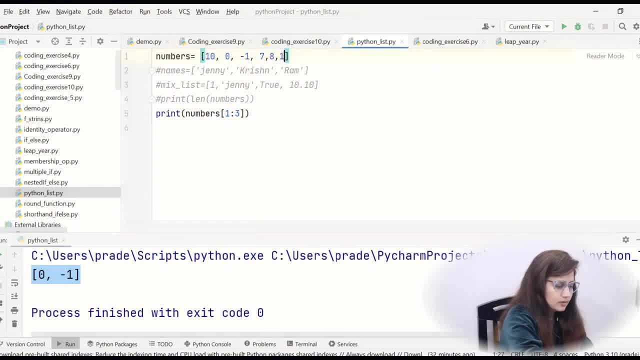 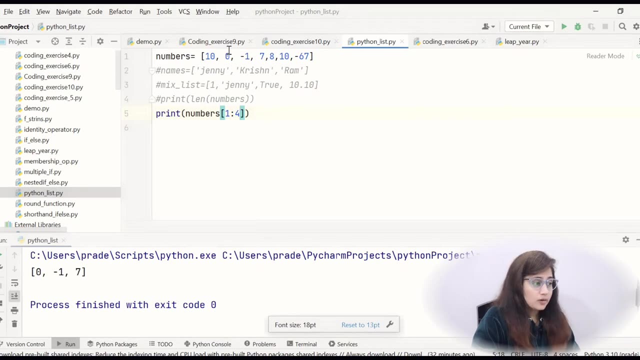 If list is something like this: 7, 8, 10 comma, suppose the minus 67.. Ok, Ok, Ok, Ok, Ok. And now if I print 1, 2, 4, so see now what it will print: index 1: 0 from 0, right, because? 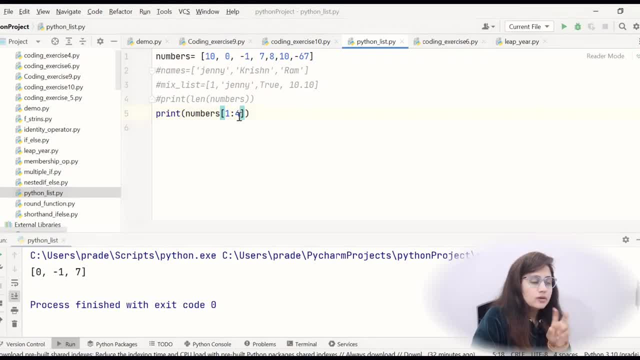 at 1th index 0, is there 0, 2. this 4 is not index, because index of 0, 1, 2, 3, 4, index of 8 is 4.. So means you think that it will print till 8.. 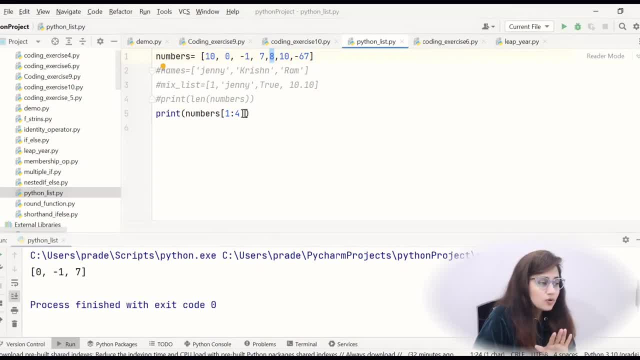 Ok, Ok, Ok, No, this 4 is what length till 4 length. this is length, So length would be started from 1, 1, 2, 3, 4.. So till 7 we have the 4 length. 4th length of the string means length 4 of the string. 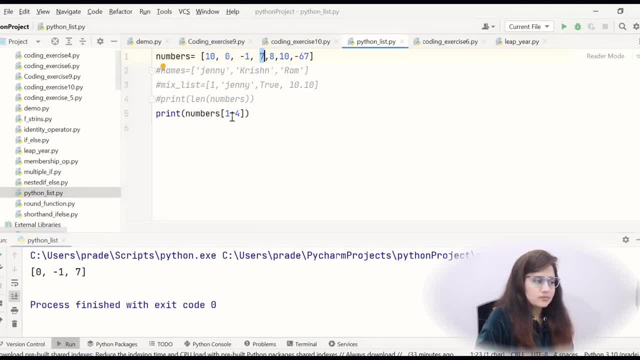 So it will print till 7 only. so 0 minus 1, 7, right. So you can say whatever you will provide here: 4, that minus 1 index it will print. Ok, Right, So means till 3rd index it will print 0, 1, 2, 3. 3rd index, 7, is having index 3.. 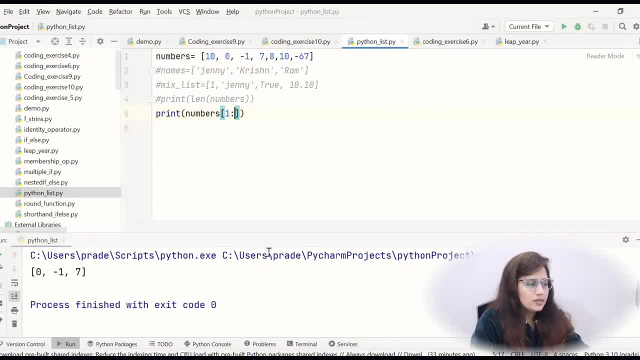 Right, So this is what string slicing, If I do not write anything here. so from starting from 0, it will print by default. last argument is: what complete length of the string? Right, And if I do not put somewhere here and if I write 5th till 5th length, it will print. 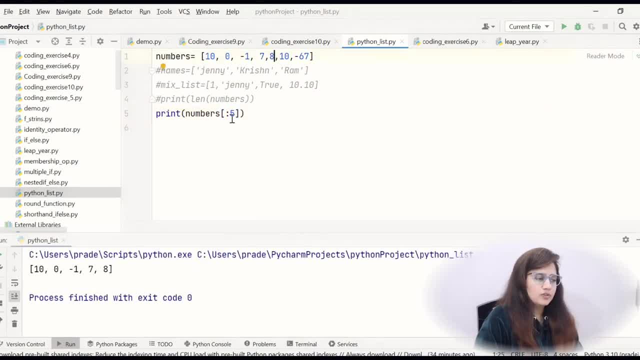 So from starting it will print till 8.. It will print till 8, till 5th length and by default it is 0. Right. But one more is what if you want to print the sub list or you can say this is what extended. 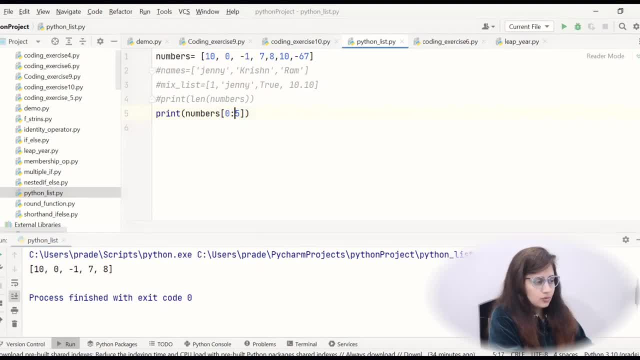 slicing like from 0 to length 5. one more colon. and third argument is the steps. Suppose I am writing here: 1. Right, So one step, it will skip and it will print the next. Right, So one step is nothing, it will skip. 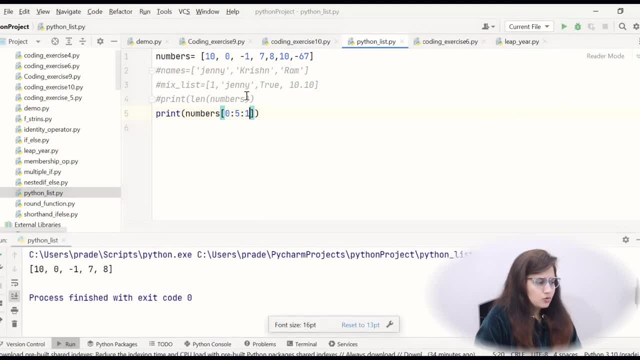 So ok, let me show you first of all From 0 to 5th length. so 10, 0 minus 1, 7, 8. Ok, But rather than 1, if I write 2 here, then it will jump 2 step. 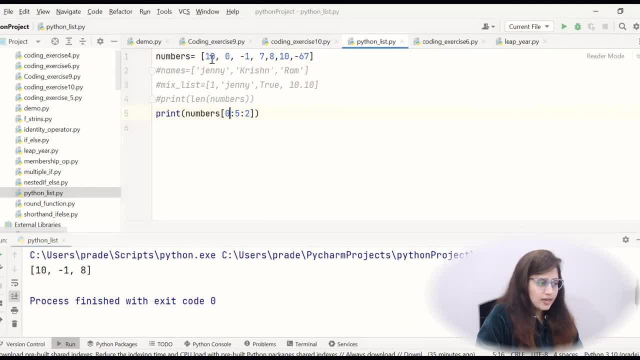 See at starting from 0th index, so 10, then steps are 2. So like from 10, 10 to 0, 1 then 2.. So 0, it will skip And it will print next element minus 1.. Then 1, then 2.. 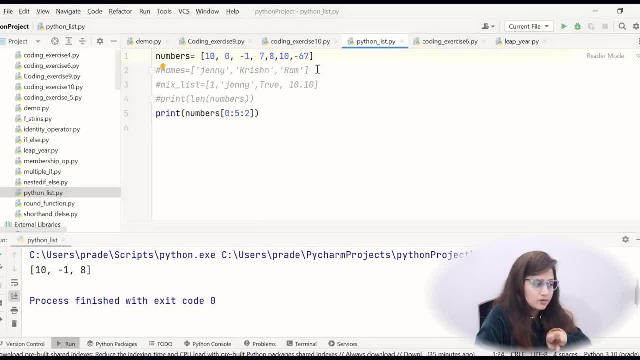 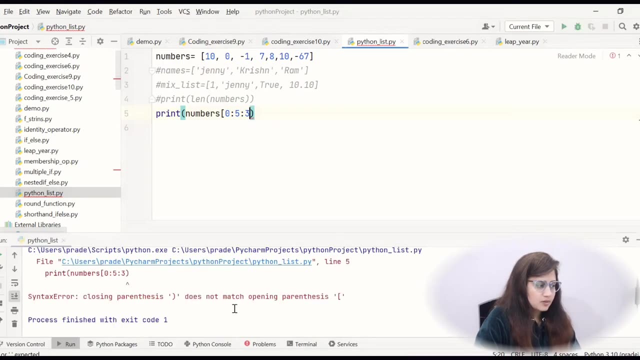 Then after second step it is 8.. So 8 it will print Till 5th index. it should print Right. So this is what extended slicing. If I write here 3, then what it will print 10.. Ok, sorry. 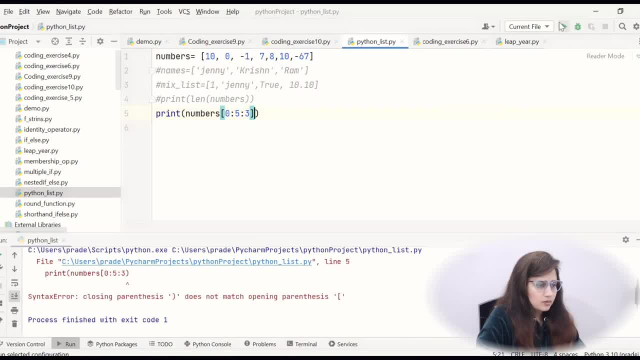 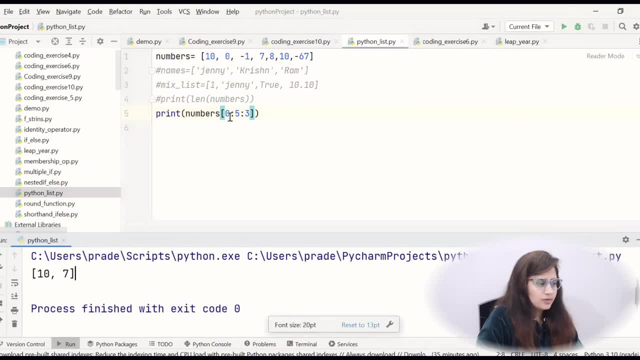 See, it will print only 10 and 7. Because it would be started from 10. From 0th index, 10. Then it will skip 2. Because 3rd step, So 1, 2, 3. At 3rd step we have 7.. 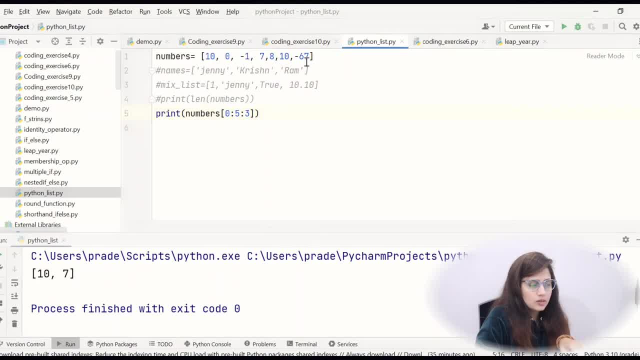 So 7. it will print 1, 2, 3 minus 67. But till 5th length we have to print. If you do not write 5 here, then by default it will print minus 67 also, Because till the end it will print. 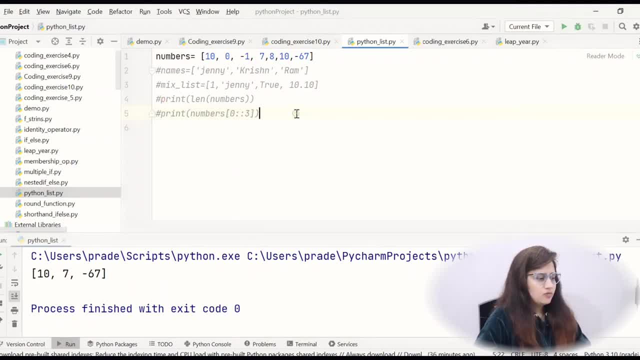 Right. So I hope you got Now some functions like: if you want to sort the list, So we can simply write what Like numbers the list name dot a function we have Sort, And then we can simply print the list Numbers. 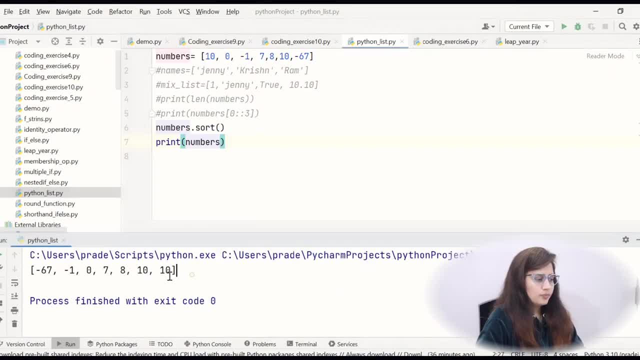 Right, Let's see what happens. That would be in sort. That would be in sorted order. Right, Duplicates are allowed 10.. 10, we have. I have told you duplicates are allowed in list, Right. But if you think directly here I can print like in 1 line only. 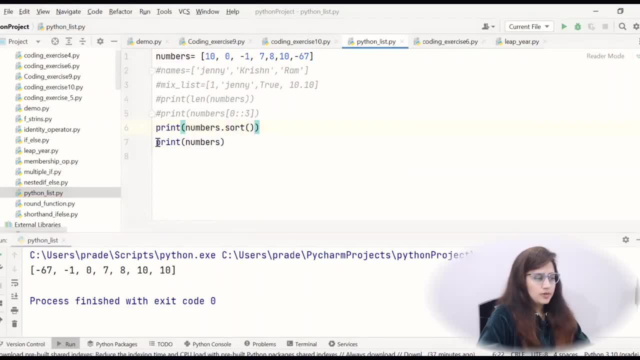 Rather than writing it in 2 line Numbers print. It will print nothing. None, it will give See none. Because this function will return nothing. No, return type Right. So we cannot do this thing. You have to sort first. 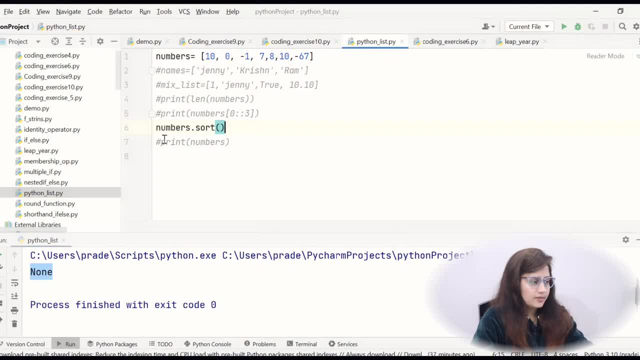 Right, And then you have to print the list, Because it will change this original list only Right Now one function is reverse. So rather than sort we can do reverse Right, And if I print then it would be reverse of the list. 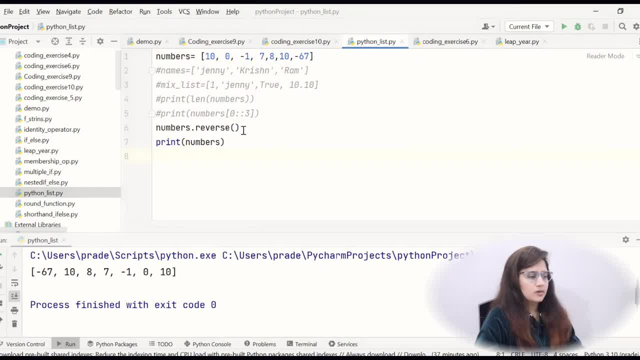 Minus 67, 10, 8, 7, minus 1, 0, 10.. So this reverse will do reverse of the list. as the name suggest Length, we can find out maximum minimum. just you can write down min and max. 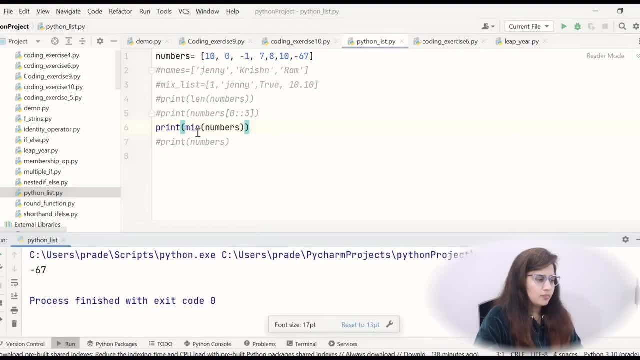 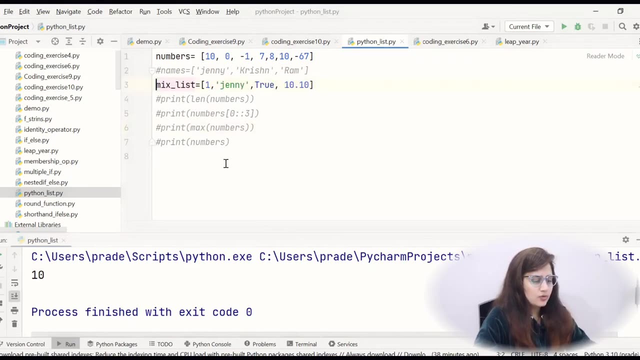 So this min function will simply print the minimum from the list. If I write like max, then max will return simply the max Max is 10.. But one thing: we cannot apply this sort on the mix list. This will give error If I do something like this. 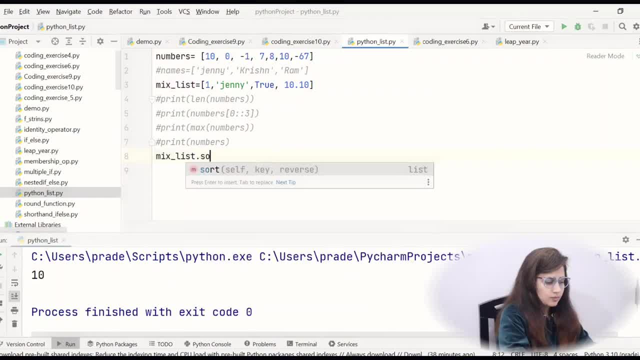 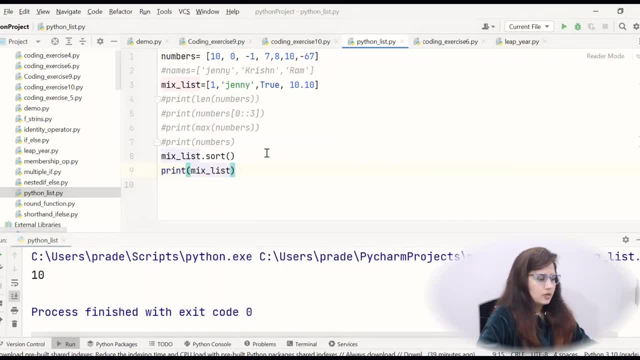 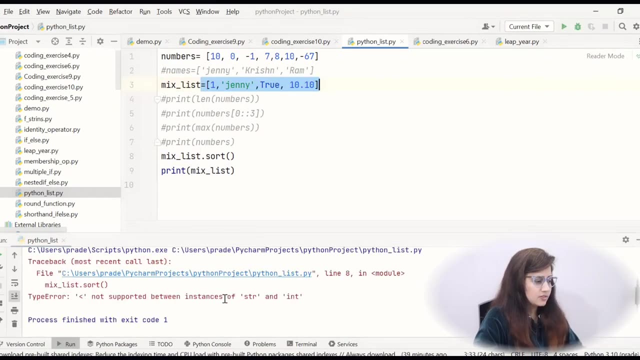 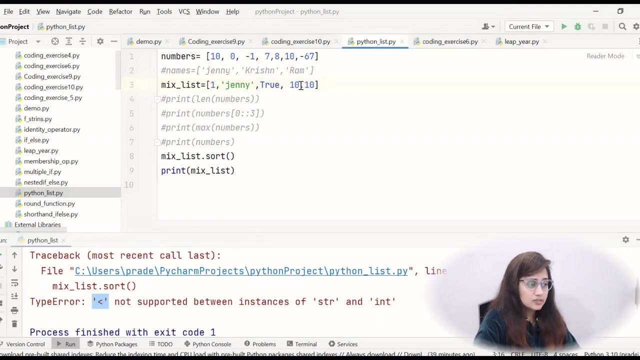 If I apply this sort on this mix list, having the list is having mixed data type And if I run this, then see This less than not supported between instance of string and int, Because this is int, This is string, This is boolean. 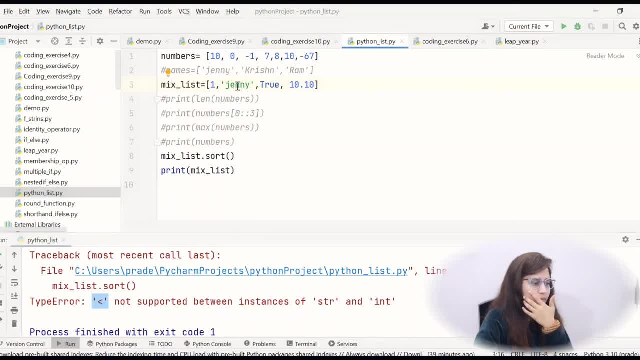 So we cannot compare different data types. So sorting on mix list is not allowed Right Now if you want to add something in the list. So there are three methods basically. So one is you can append. You can use append. Append means at the end of the list. we can add one element at a time. 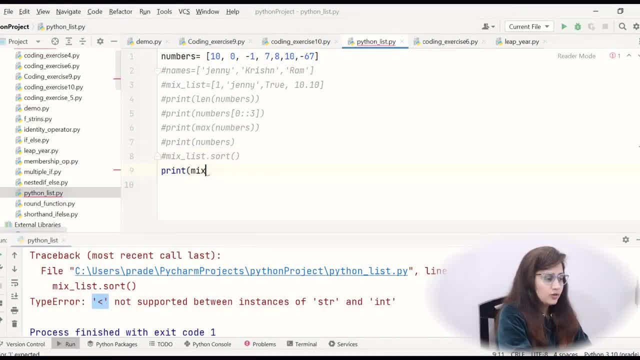 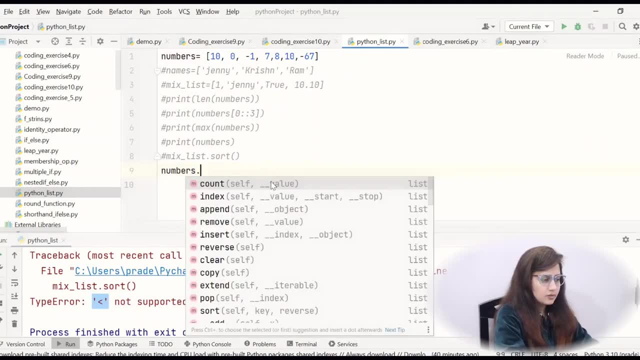 One element at a time at the end of the list. if you want to add, Then you can use append. So how you can use that thing? just This is the list: Name of the list, Numbers, Then dot, Then append And the value. 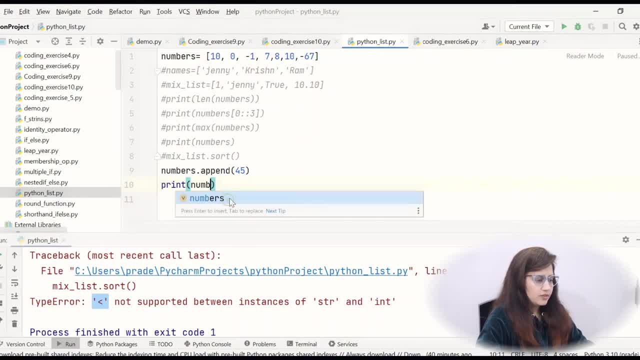 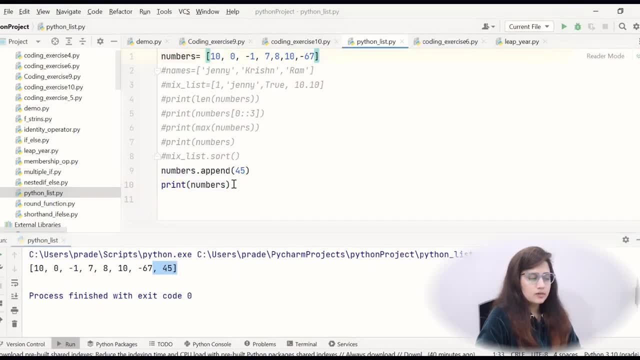 What you want to add: Forty five, And after that I am printing this numbers, So let's run this. See now, Forty five is at the end of the list. Right, One more. append you can: Forty six, Forty seven. 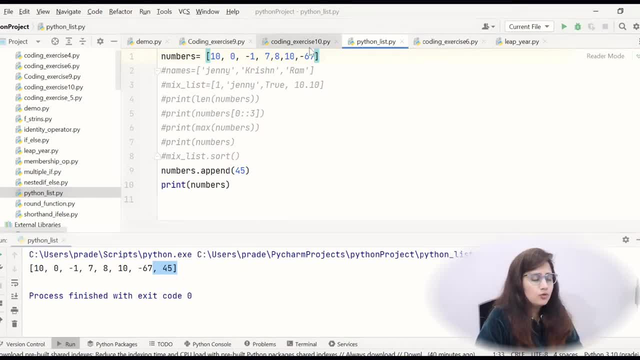 Like this: These would be added at the end of the list, But at one element at a time. So, generally what we do: We create a sing, You know, Empty list Like numbers, Just the brackets, Nothing, And then we append the numbers. 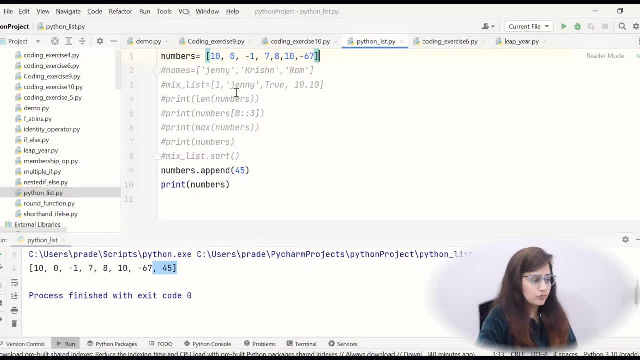 Right In the list. That also we can do So. next is: You can insert, But at specific position. I want to insert a data, Not at the end Specific index, Like at second index, Third index. Then we can use insert function. 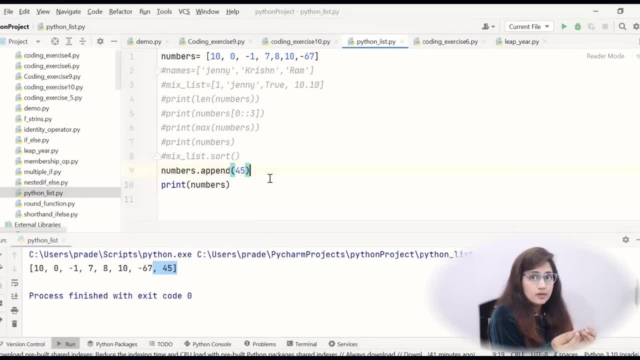 So here what we can do Like numbers, rather than append, We can do insert, But in append we pass only one argument: The value you want to add. But here you will pass two argument. First argument is At which index you want to add. 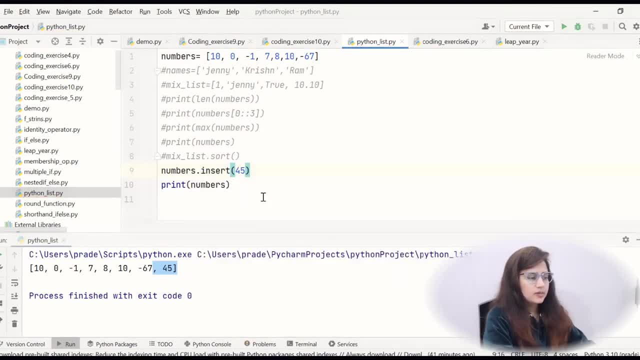 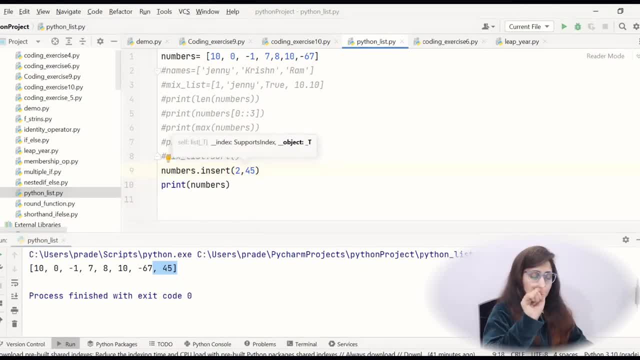 Right Comma What you want to add: Forty five. I want to add, at Second Means, zero, One, Two Means. here At second index, Forty five would be added And This would be shifted to Right side. 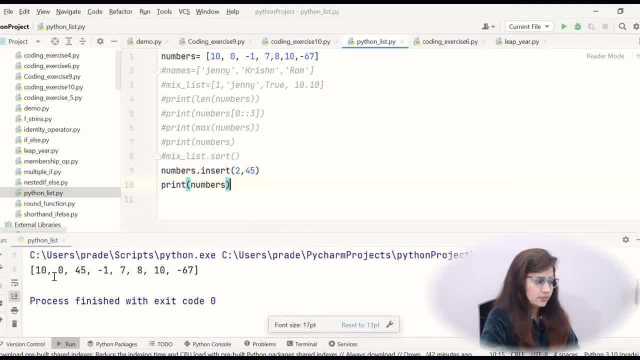 All the Data. Let me just run this And that you, Then you will get it better. See Ten, Zero, Then forty five, Right At second index, Then minus one, Seven Eight, So You can replace. 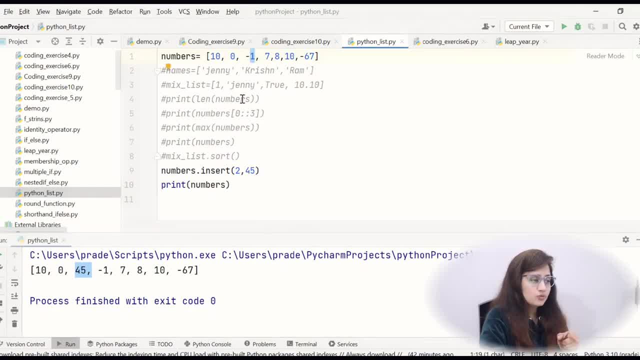 This minus one, Because at second index minus one is there. Maybe you will think It would be replaced with forty five. No, It will add forty five Minus one would be still in the list and would be right shifted. So this is how, at particular position, you can insert: 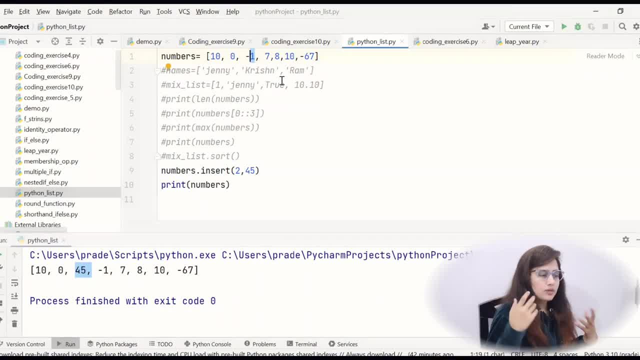 One is: If I want to Add More than one data at one at same time, Right Then, Using append, we can only add one data. using insert, also, we can. at one time, we can add only one data. Yes, We can use insert, insert, insert two to three times if you want to add two to three items. 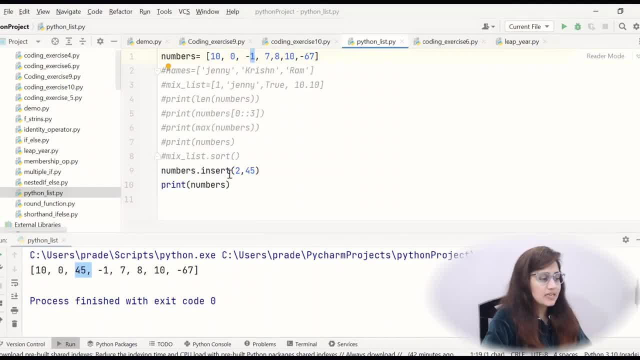 But at the same time you want to add three items, then one function is extend, So that you can do Extend And in bracket now we can pass list Like I want to add: forty five, forty six, forty seven, seventy, eight, eighty, nine, This list I want to add. 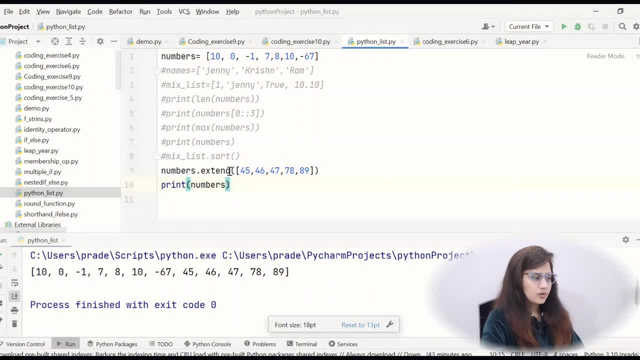 And simply we just print numbers. Now see This list now extended At the end, After minus sixty seven, forty five, forty six, forty seven, forty seventy, eight, eighty, nine. This list would be added More than one item, but At the end of the list. 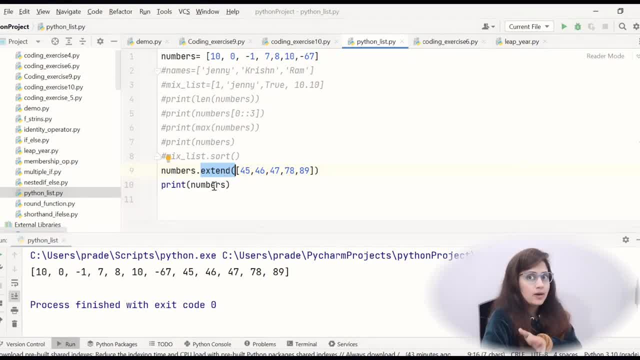 Extend also add at the end of the list More than one item. Append will add at the end of the list at only one item at a single time, at one time, Right? So this is what extended list now Right? One more thing, what we can do, like if you want to change. 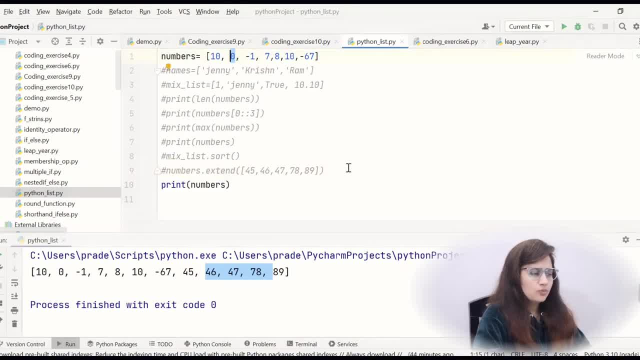 Like: at first index I have zero, but I want to change the zero. So what we can do Like numbers, name of the list. Then at which index you want to change the data? First, index, What you want to insert. now, rather than zero, I want to insert, suppose, forty five here. 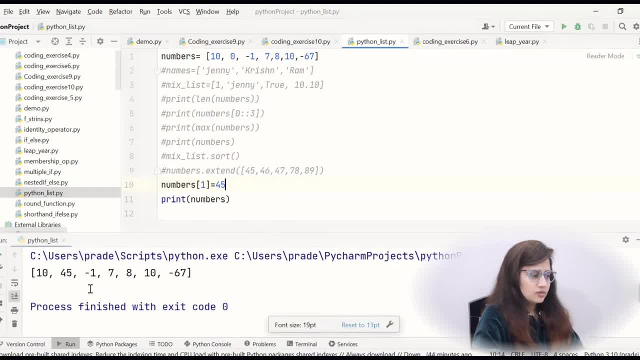 And now I will print numbers. So this At the place of zero: now I have forty five, Forty five in the list, Right? So this is how you can change the list. So that is why I have told you list are mutable. 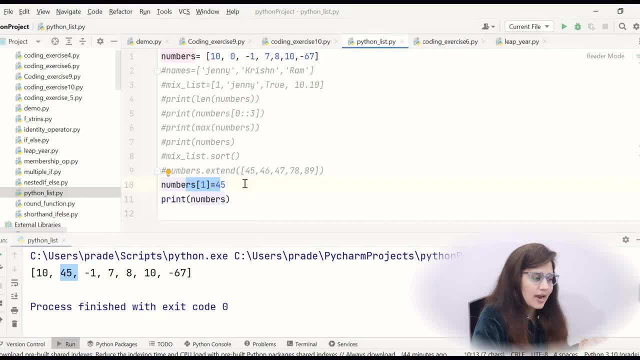 We can alter the list. after creation of the list. We can add, change the data and remove and remove the data. Now I want to remove something. Okay, Now one more thing, If I want, if I do something like this: Index one, two, four. 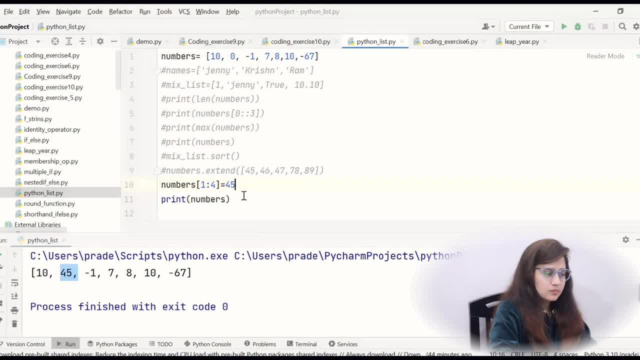 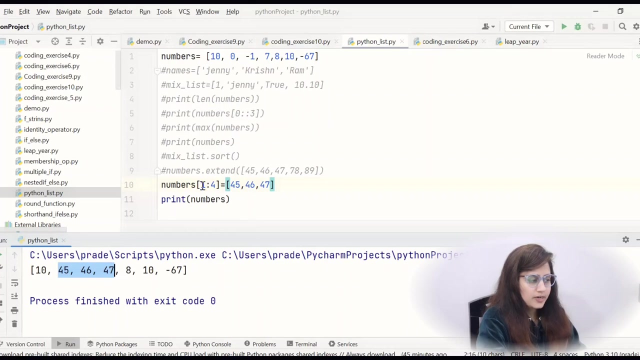 One, two, four. One, two, four means one, two, three, Three element. I want to add: So, if I do something like this, forty five, forty six, forty seven, Now what will happen? See, These three elements from the index is one and this four is what. 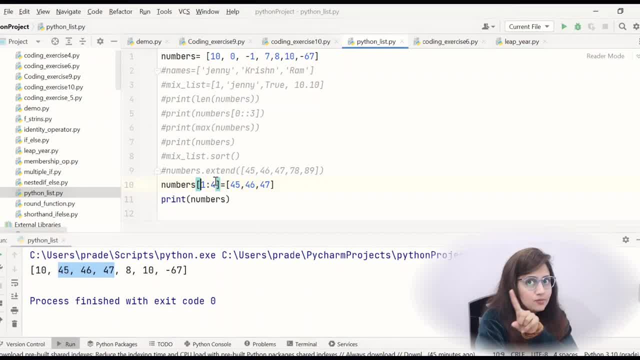 Not index. This is length Till fourth. length Means till index. this length minus one till third index. So it is first index, second index, third index, Forty five, forty six, forty seven rather than zero minus one and seven, And all the other elements would be same. 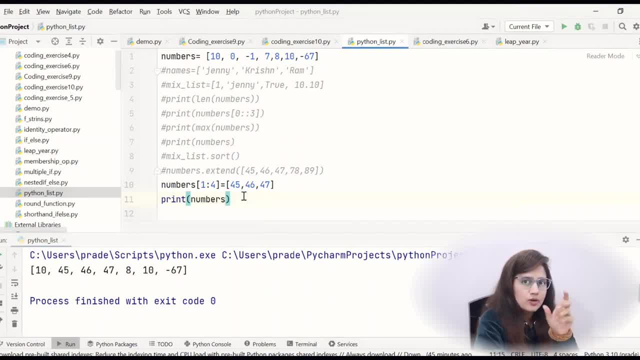 Right, So you can modify more than one item also. You just have to provide the range where you want to modify Right Now. if you want to remove something, then we have two methods: Remove as well as pop. Remove will search the item and just remove. 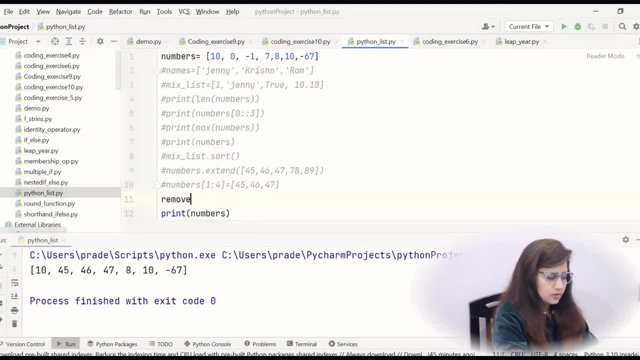 It will not return anything. So like sorry, first the name of the list, numbers, dot, remove, and in bracket will pass the value, the item you want to remove, Right? So suppose I want to remove zero from this, This list, So let's run this. 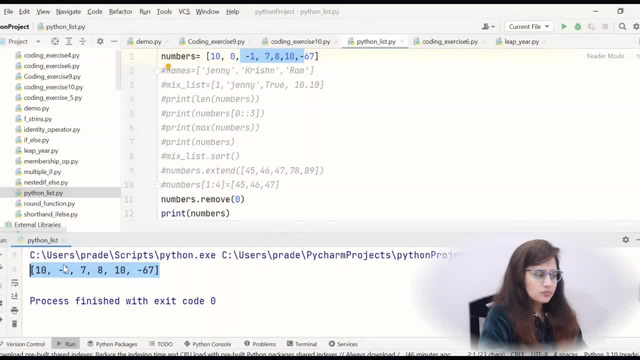 See, Zero is not there now. See, maybe you are thinking we have modified this list here like extend and all, But I have just commented out these line. So original list is now this: Right, And on this only I am performing this remove operation. 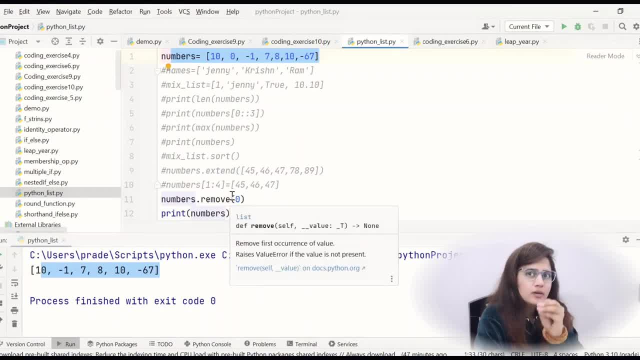 So it will not return anything. It will just search the item and remove. But it will remove the first occurrence of that letter. Suppose, here I have one more zero, Two zero are there, And now I am removing zero. Let's run this. 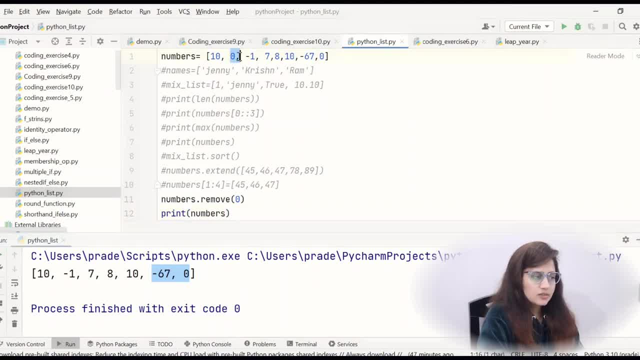 But still in the list we have zero, But first occurrence It will search from starting. It will find zero here. It will remove zero and it will print the list. It will not remove this zero. Remove will remove only first occurrence of that letter. 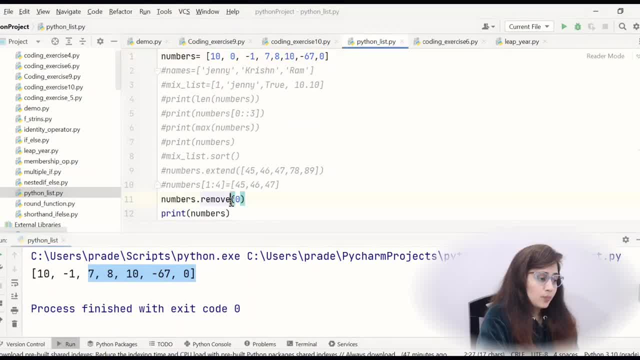 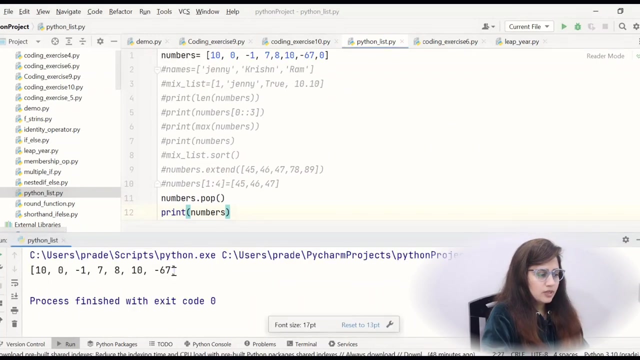 Right Now: Pop Numbers, dot, pop, Yeah, It will return What pop means: It will chop off the remove the last element by default, The last element of the list. So if now I print numbers, then see Now, then there is, the last zero has been removed. 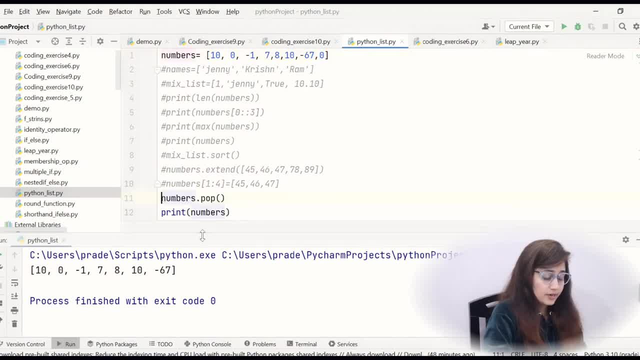 So pop will remove the last zero And if it will remove that, it will remove as well as it will return that element. So if I want to print what this pop has removed from the list, So it will print that element, So it will print that element also. 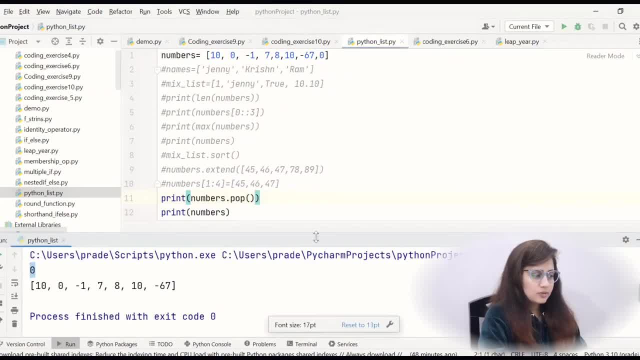 It will return that element. See, Zero. Zero has been removed and after that we have printed the list Right. But if you want to remove specific element, then you just pass the index in this pop. Suppose I want to remove not the last zero. 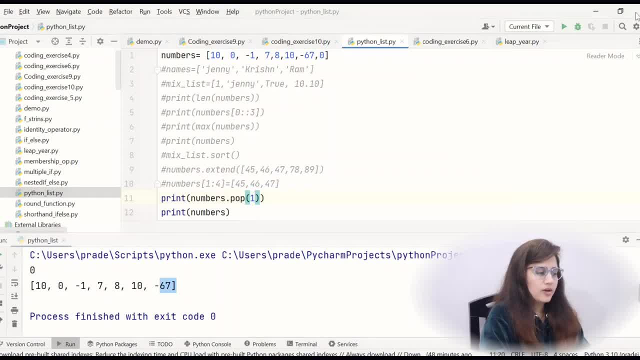 This zero. So index of this zero is one. Now let me just run this. See Now it has removed zero, but from first index Last zero is as it is Right. So just pass the index. If I pass five, So it will delete this five. 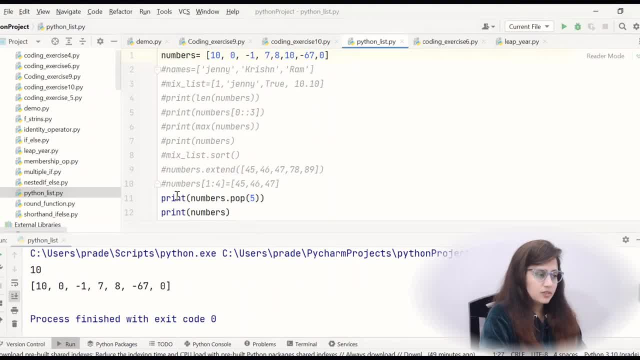 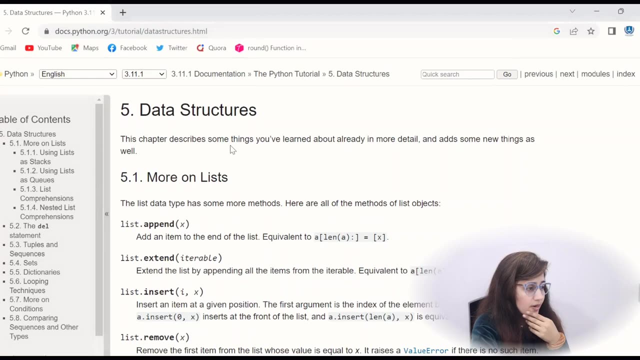 This l, This ten At the fifth index. This ten is there, So it will remove this and it will print the list. So this is how pop will work And there are many methods. See, as you can see here, This: this the python documentation of python. 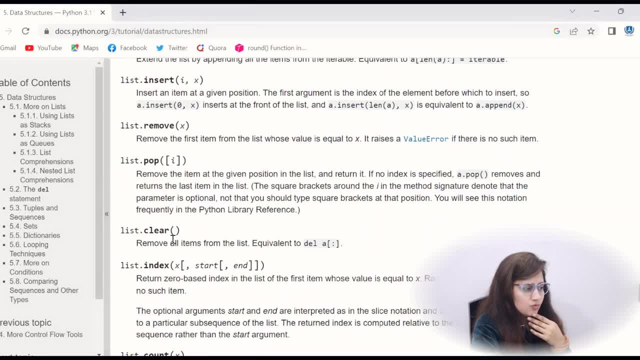 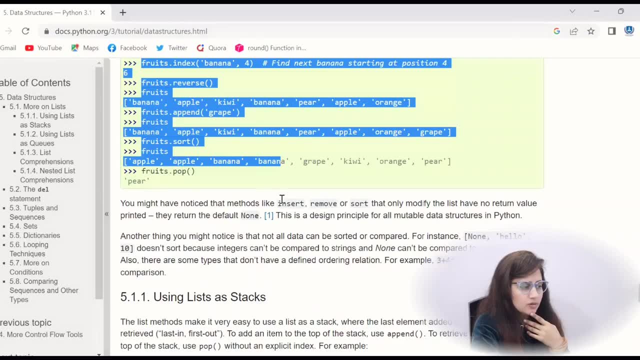 Here there are many methods Like append, Extend, Insert, Remove, Pop, Clear, Index, Count, Sort, Reverse, Copy And how to use these methods with one example they have given, So do not have to memorize these methods. 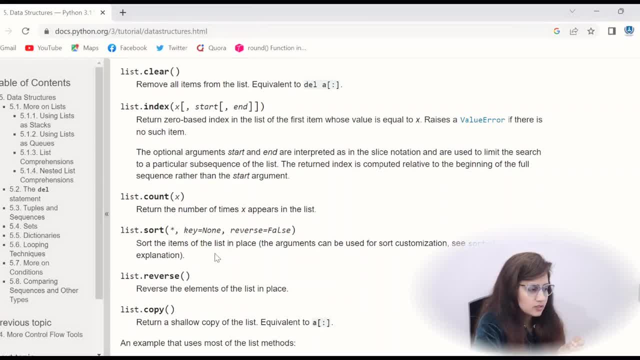 You can just search, But you just have to go through these methods. Yeah, We can. Can you reverse a string? Then you have in your mind, Yes, You should know you can reverse the string, and then how to reverse that. you can simply.